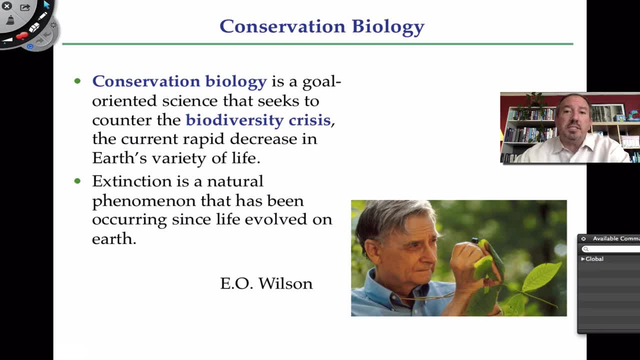 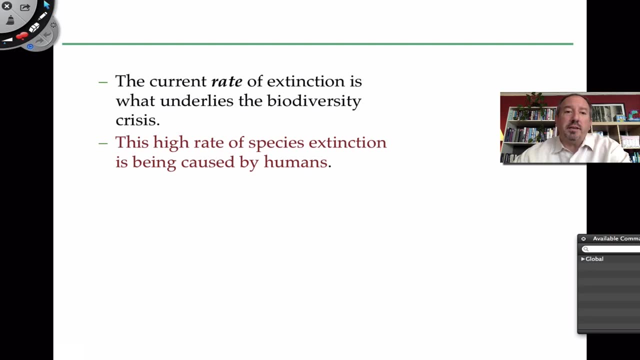 about three and a half billion years, And so we've seen extinction before. We know that it occurs from the fossil record, but it's occurring this time in a really rapid event, And the reason being is that it has to do with one species in particular, and that's humans. 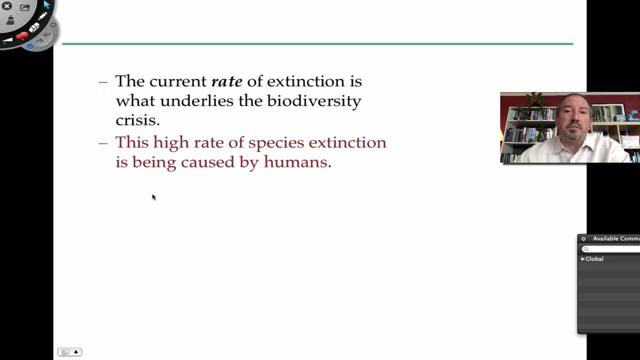 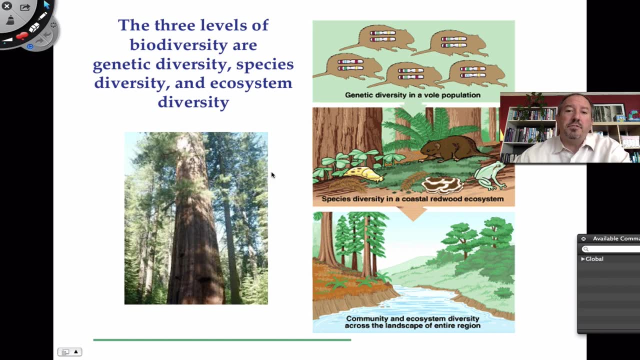 It seems that humans are being the cause of this rapid extinction, And so if we're the cause of it, we have to take responsibility, to sort of: you know, stop that. And so biodiversity can be studied on three different basic levels, And so one of the levels, the largest level, is what? 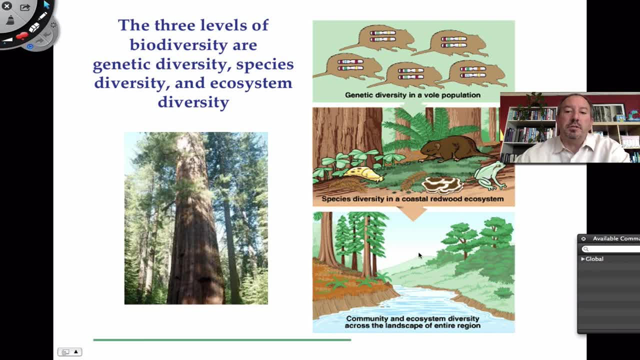 you'd call community and ecosystem diversity. So in other words, you want to protect like a redwood forest, because by protecting the redwood forest you're really protecting the ecosystem, And so you're protecting all of the organisms that are living inside of that forest. You can also protect 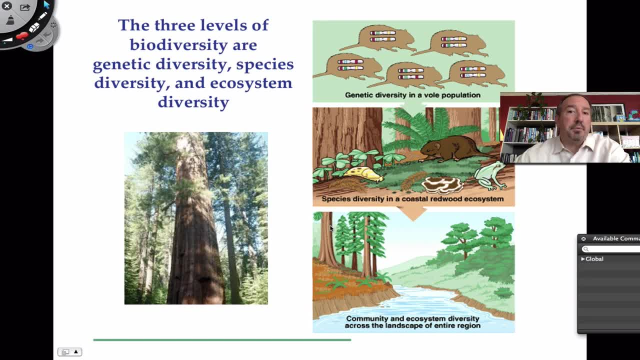 the tropical rainforest, You can protect the chaparral, You could protect the coral reefs of the world in the ocean, And so these are particular areas of hotspots that are crucial because there's a lot of species diversity in there and they're essential, So you can go. 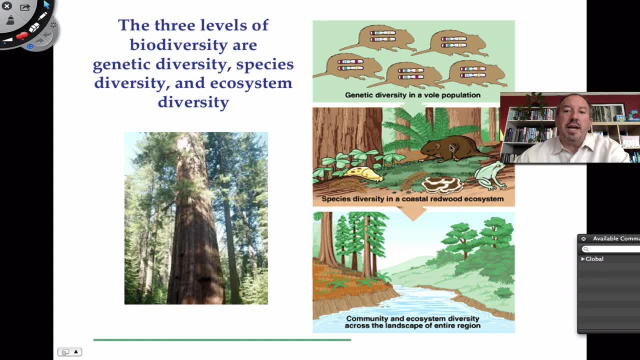 at it that way. Or you can look at protecting individual species, And so the species diversity is rather important too. So you could try to protect: save the redwood, protect the redwood, swirl the fern or the frogs, banana slugs- You can look at species. 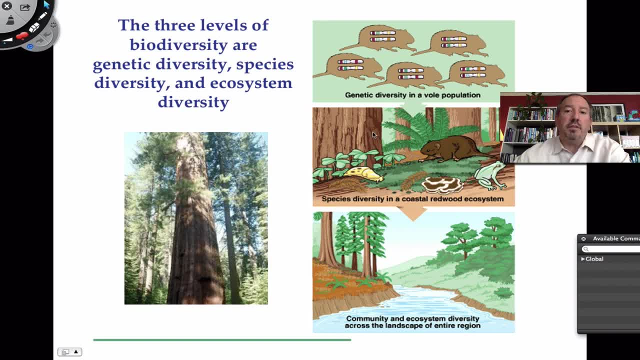 protecting them individually, Okay, And that's important too. Or you could look at within a species, like, for example, within the vole population. genetically there's diversity there, And so the greater the diversity, the greater the diversity, And so the greater the diversity. 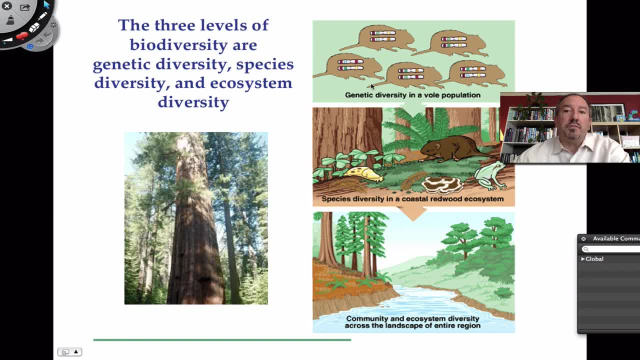 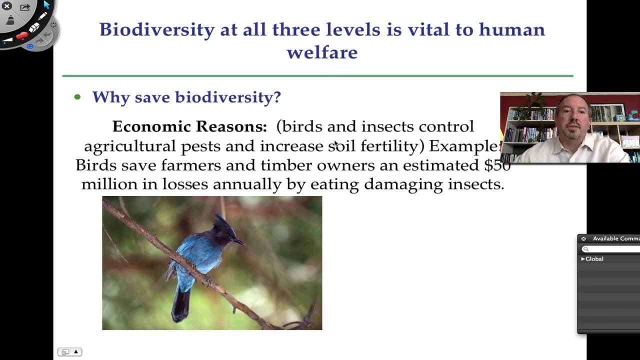 within the population, the better the whole species is going to be doing, Because, again, genetic diversity is rather important in terms of survival, to withstand sort of threats to the species in terms of like, for example, disease is an example of one of those, And so you know. 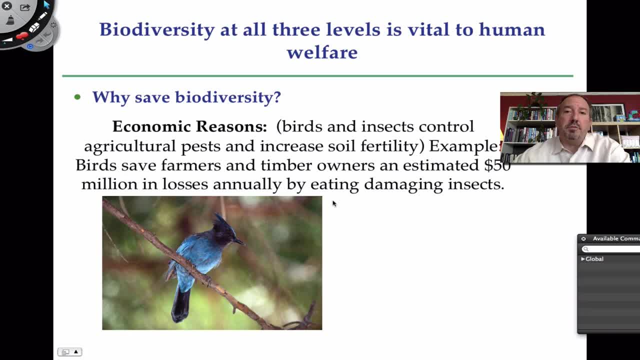 why would we, why would we care about protecting biodiversity? Well, I mean, if you turn, turn it upon ourselves and make it sort of human centric. it, our own welfare, is dependent on biodiversity, And so I mean it's worthwhile to protect in and of itself. 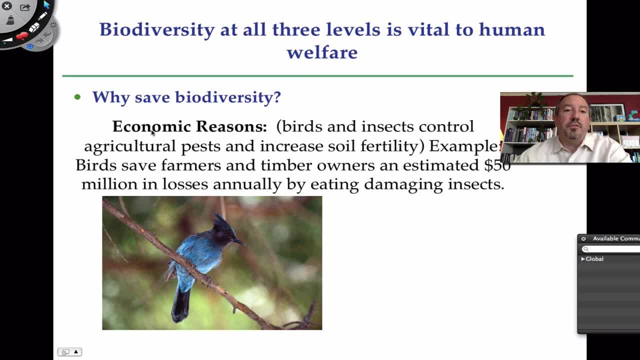 but I'll just turn it into human centric for a second. So for economic reasons, we want to protect biodiversity, Like, for example, just having a lot of birds and insects and a diversity of that will help to reduce birds, help to reduce pests that are attacking our crops, And so 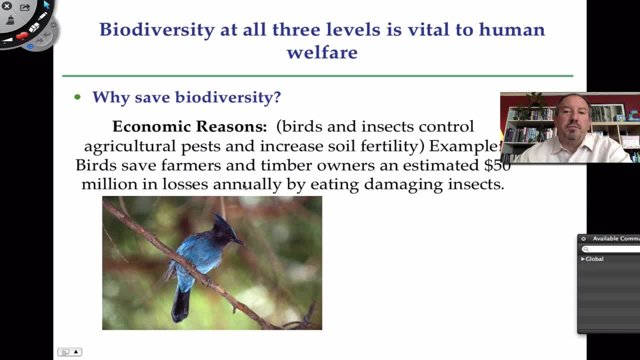 birds alone save farmers millions of dollars that would be otherwise lost to insects, And so, for economic reasons, we need to protect biodiversity. I mean, this is really on a large scale. this is really important to some countries like, for example- I'll just throw it out- Costa Rica in. 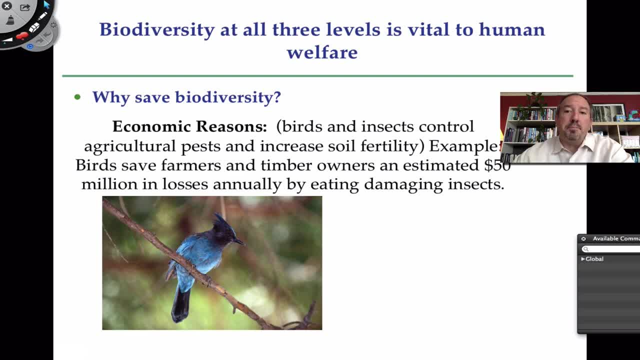 Central America. It's really economically important for them to maintain their tropical rainforest for ecotourism, So it's valuable to not disrupt biodiversity, And so you know we can't, you know we can't just interrupt those ecosystems, And then this is a huge one for. 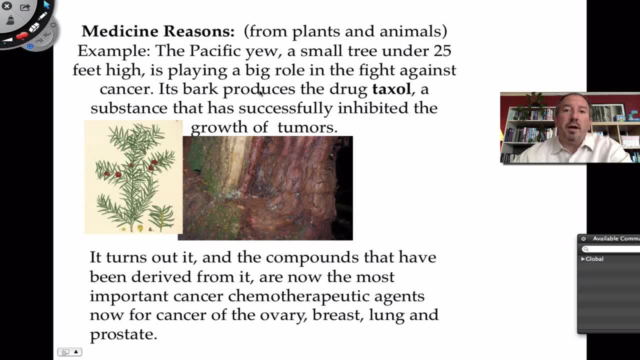 medical purposes. You know, we get a lot of our pharmaceuticals and therapeuticals from plants, And so it's very difficult to come up with these medicines in and of themselves, And so we could sort of discover, either by design or serendipitously, we could discover- some important drugs that 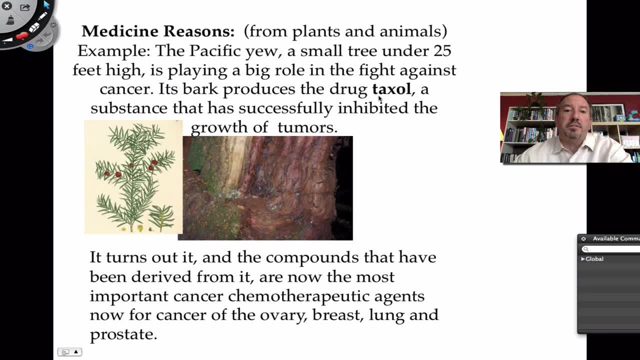 could fight off, for example, cancer, And a good example of that is something called Taxol, And Taxol came from isolating this really interesting ring structure from the pacific yew tree, and so, as it turns out that that is a really important medicine for fighting off cancer, and it's important for 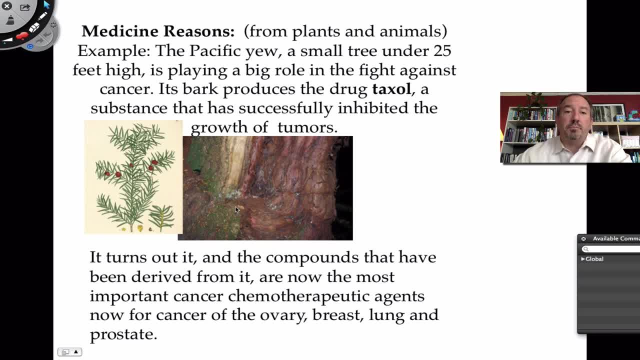 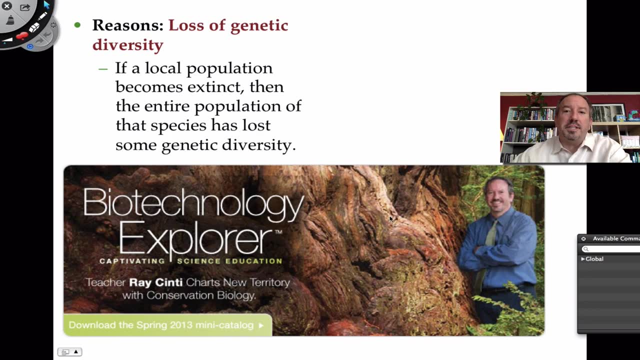 like ovarian breast cancer, lung cancer and prostate cancer, and so it's really critical: if we lose trees, we could possibly lose cures for future diseases and ones that are with us, and so we're really curious about this, and so, if you don't mind me indulging a little bit on 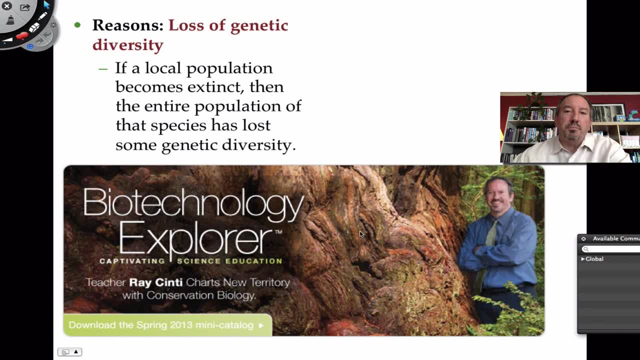 something personal, but i have the the privilege and fortune to be able to teach a class on conservation biology, but it's really a biotechnology class in disguise, because we're, instead of just going over the principles of conservation biology, we're out there doing it. we're out there protecting species, and what we're we're looking at is we're studying genetic. 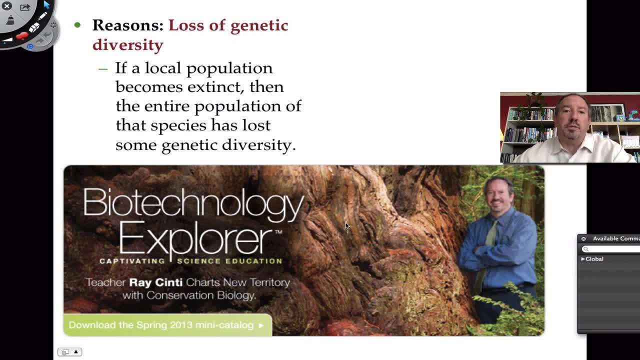 diversity. we're studying it within the population of coastal redwood trees, and so, again, what we're doing is we're isolating dna from these trees, we're crushing down the needles and we're analyzing to see how genetically similar members are in a particular grove, because the more diverse 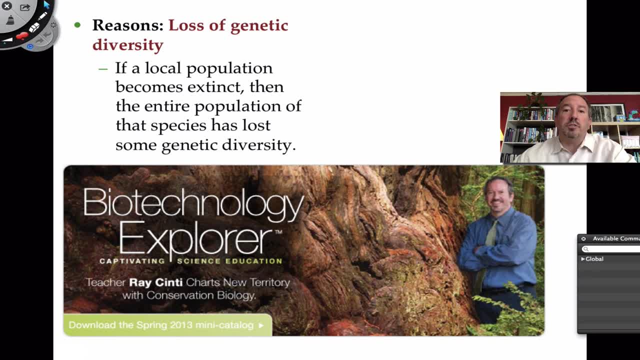 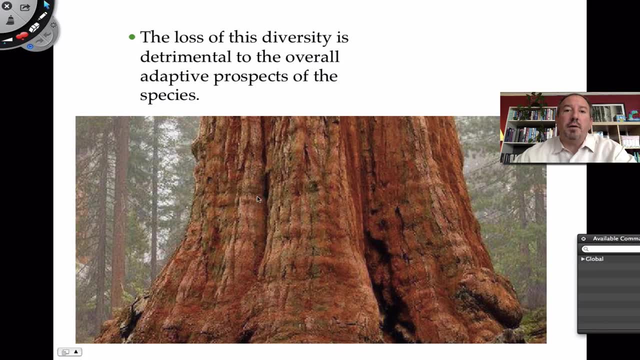 we're thinking, the better that population will be in order to survive climate change or an invasive species or disease. so we're studying these populations of redwood trees, and so the loss of the genetic diversity of the tree is important, not only to protect the redwood, but again the redwood's sort of like an umbrella. 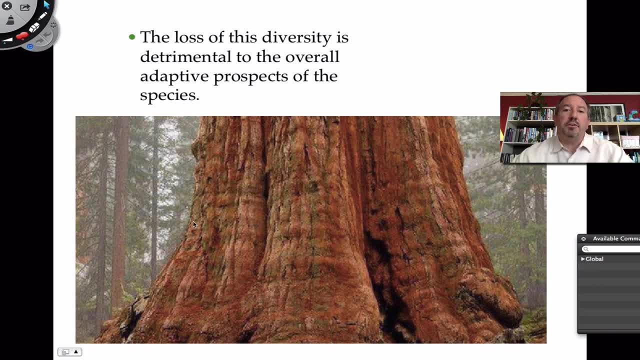 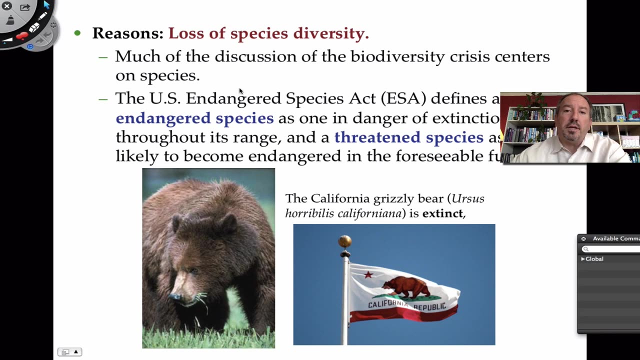 it protects everything within it. so you save the redwood tree, you really save the entire community. so it's extremely important. so i'm fortunate to be able to be researching in this area, and so the loss of species diversity is really important again, not only just the 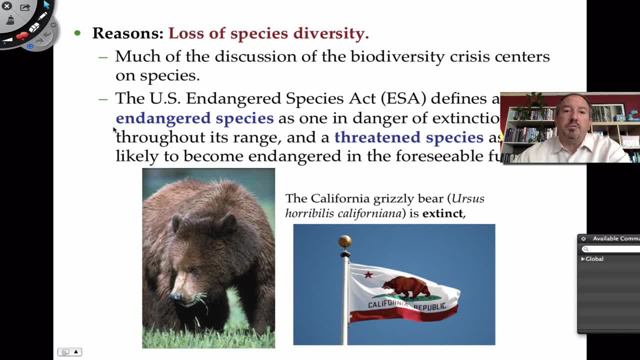 redwood trees, but it's important for all species to be preserved, and so the united states is actually entered into this conversation. they've they've come up with the endangered species act- i'm not sure if you've heard of it before, but maybe you have- and so we can start to classify. 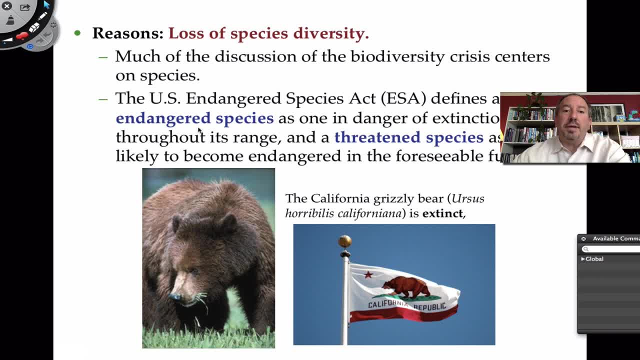 organisms based on their number, as either being endangered- in other words close to going extinct- or threatened, meaning likely to become endangered in the foreseeable future. and so if you look at the, if you look up a particular organism on wikipedia, it'll actually give you as their status in terms of if they're threatened or if they're endangered or if they're doing okay. it's kind of interesting. just an example: locally, i mean, this is our the california grizzly bear. and you're like: wait a minute, california grizzly bear. i didn't know there were grizzly bears in california. there used to be. they're extinct in california. fortunately, they're not extinct. the population in california is extinct, but they're not worldwide. 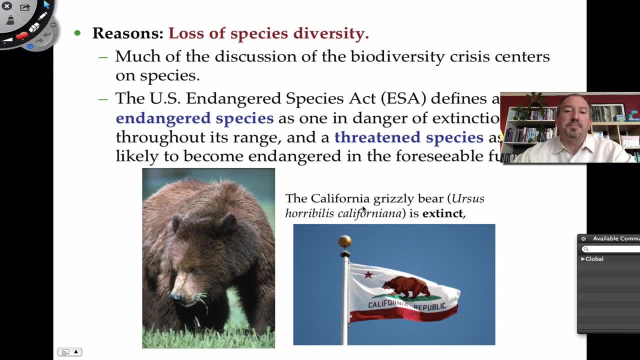 extinct, fortunately, but the california one is, and so you know, i mean you might say, well, you know this is good because you have to consider, you know, the human issues involved and so obviously the grizzly bear would be a threat to to human population. but overall i think it's really a sad state when 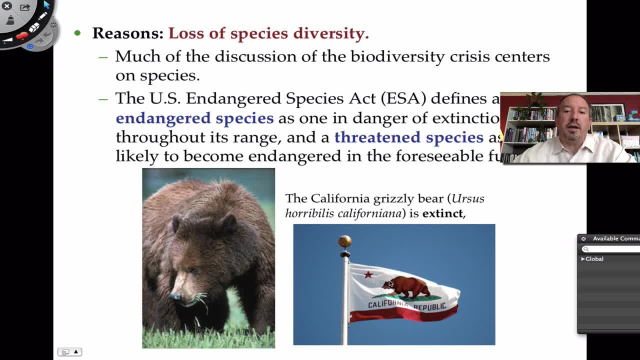 the california flag is actually flying the- uh, the grizzly bear, and it's extinct. when i look at the flag to me it's a flag telling me to step up. it's telling me to it's a reminder of the tragedy of the bear. and so did you think about that? when you see the bear flying in the flag, that it's. 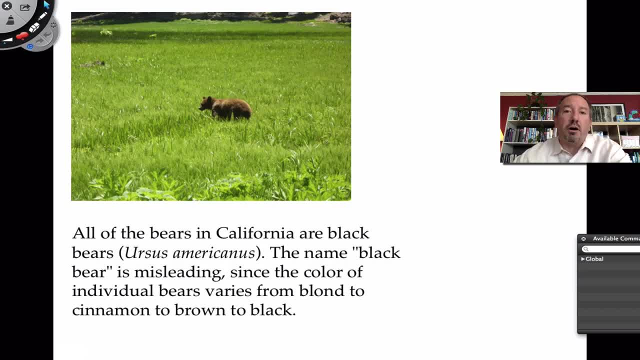 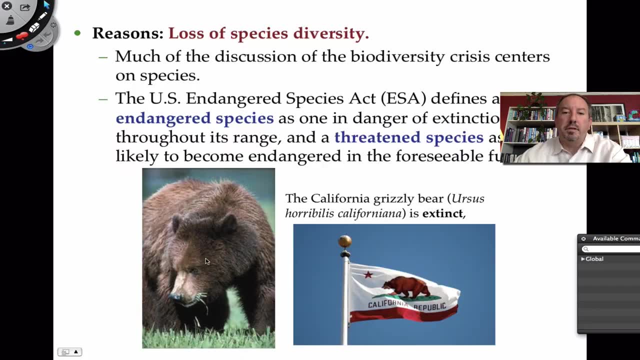 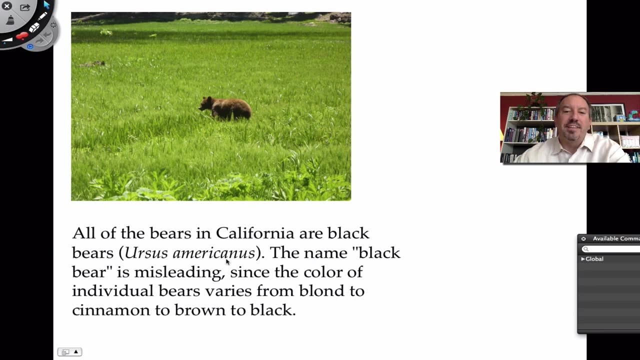 really extinct. now, not all bears in california are extinct, like um, for example, the ursus americanus, as opposed to the, the ursus- horrible, horrible, horrible. mispronouncing that, uh, the black bear. it's kind of misleading because some of them are black but some of them can be brown. 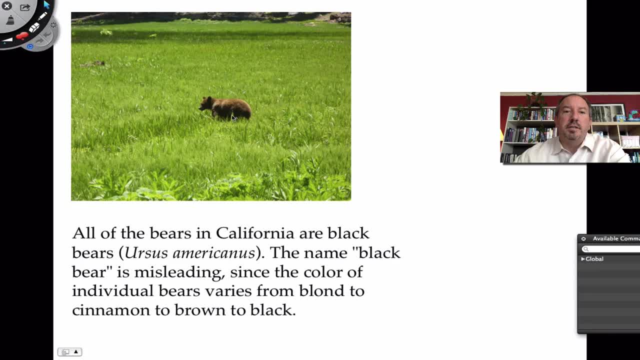 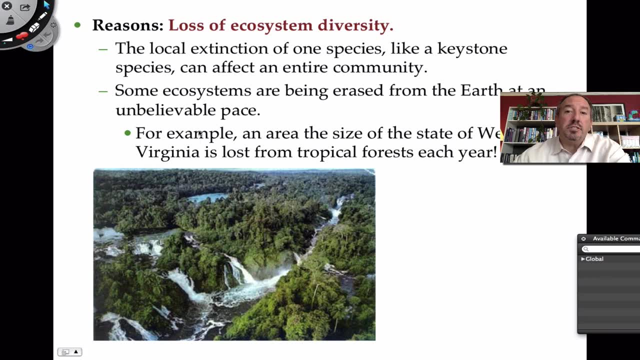 and some of them are even blonde or cinnamon color, but there is a picture of uh, of the black bear in sequoia national park, and so the loss of ecosystem diversity is a reason to protect biodiversity as well. and so, again, if you protect one species like the redwood, or if you protect something like 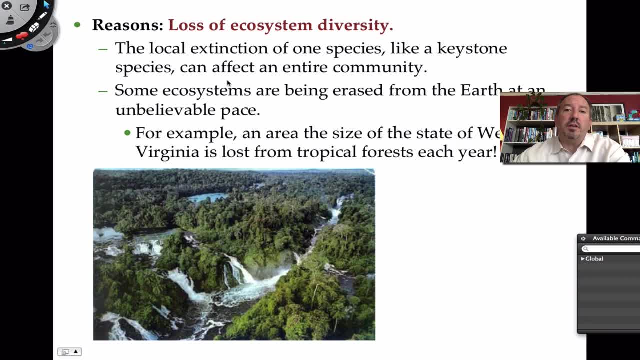 a palm tree in the tropical rainforest, it can really affect the entire community because it could be a keystone species, which means that a lot of other species depend on it. so it's rather critical for maintaining species diversity in general, and so the tropical rainforest is. 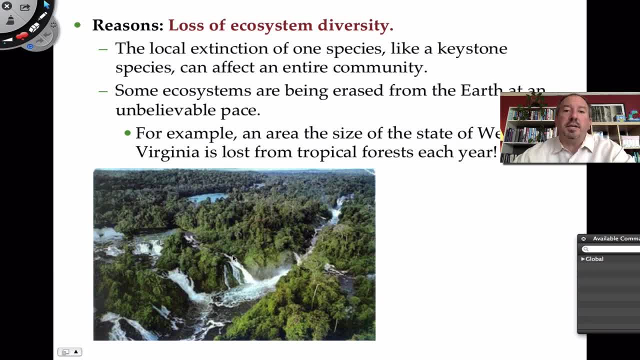 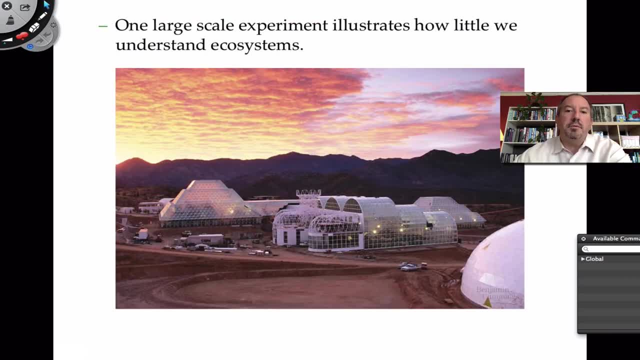 extremely critical. it must be protected and it's being obliterated. you, um, it still continues to to occur. it's brutal, and so how do we know what's going on in ecosystems? it's really difficult to study. just want to point this out. um, there's these structures in arizona. 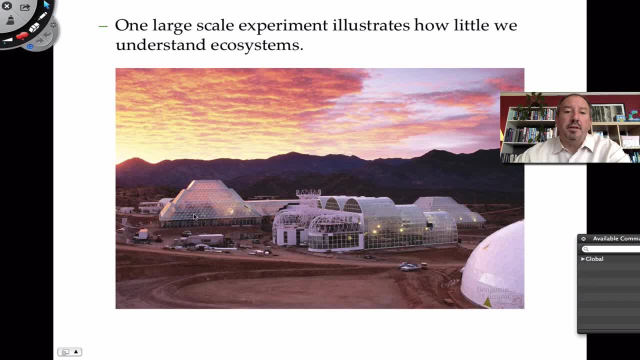 in the united states called biosphere and what. what these structures? they sort of look futuristic, but inside of them there are forests, there's little oceans in here, there's little biomes inside, and so scientists come here and they do research, and they do research, and they do research. 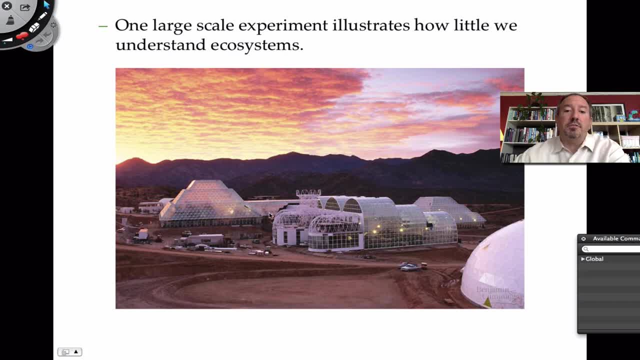 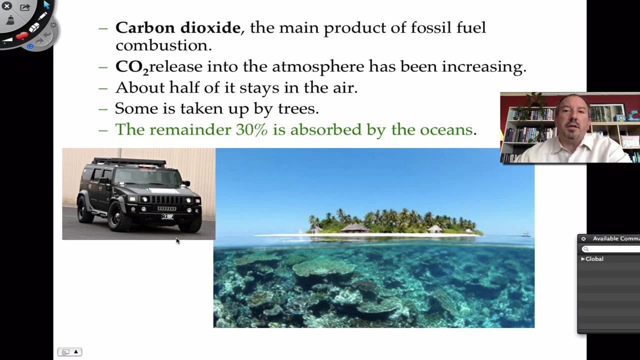 in a, in a controlled environment, meaning that it's closed off, and so they can measure things like temperature and and levels of atmospheric carbon dioxide and oxygen, and so we're trying to understand the balance between organisms. it's difficult to do it, and so one of the um interesting 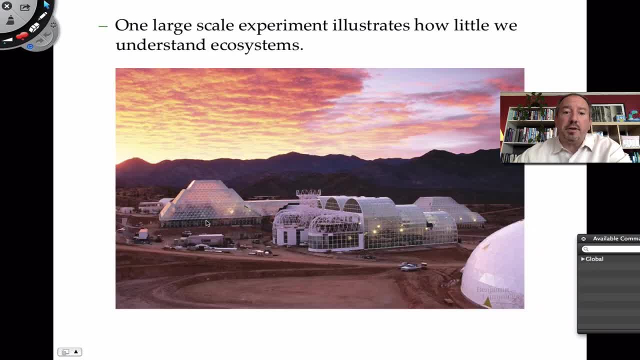 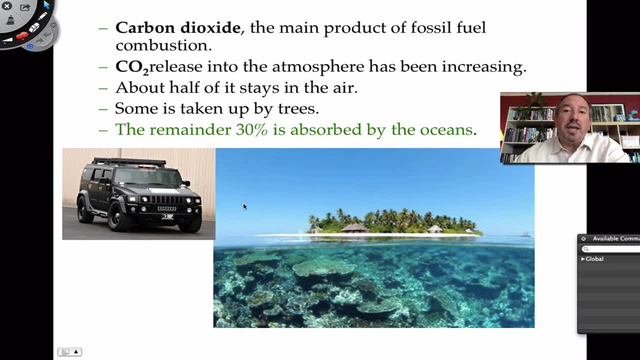 studies that is happening inside the biosphere is in the ocean biome, so this section over here is the ocean, and so, as you may know, there's a lot of research going on in the biosphere and there's a lot of. you know, the carbon dioxide is rising in in the atmosphere as a result of humans increasing 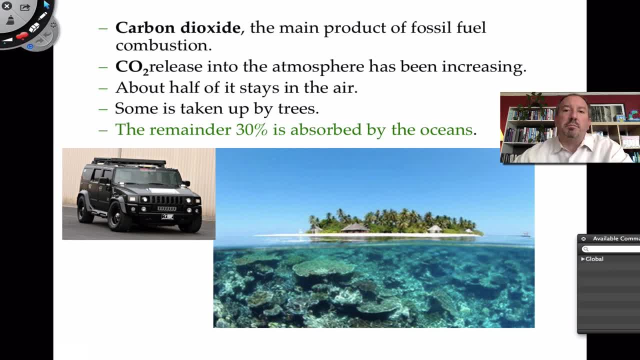 use of fossil fuels and combustion produces a lot of carbon dioxide and so that's increasing into the atmosphere. most people, when they talk about increased carbon dioxide in the atmosphere, talk about the effect that that has on climate. in other words, it's warming the planet. the more carbon dioxide because it provides insulation to the 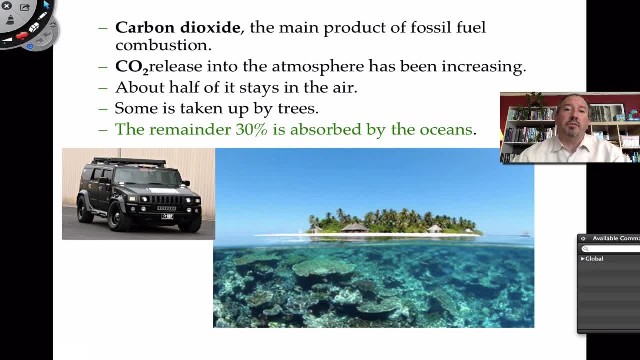 energy produced by the sun when it comes in, And so it's something called the greenhouse effect. But people sometimes forget the fact that carbon dioxide can be absorbed in the water, And when it's absorbed in the water it reacts with water, So carbon dioxide goes in the water and water. 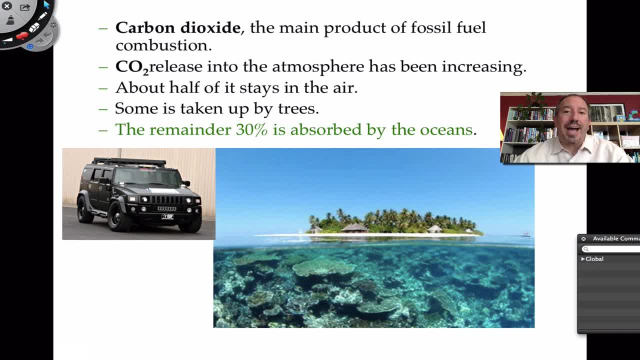 holds quite a lot And it forms something called carbonic acid and then ultimately bicarbonate ion. But what it does is it increases the acidity in the ocean, And so a lot of it is carbon dioxide, is taken up by trees for photosynthesis and also phytoplankton. 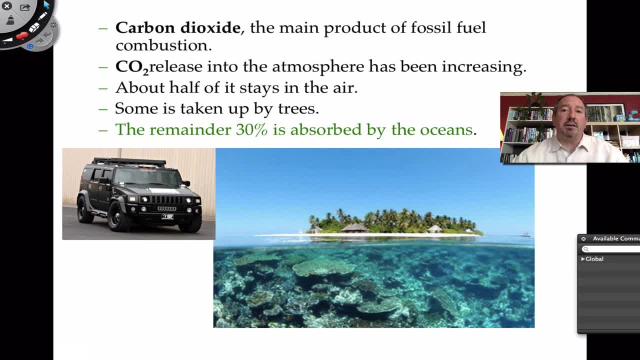 But the thing is, if humans are cutting down and deforesting trees, that's going to reduce the tree's ability to remove it from the atmosphere, And then also it's being absorbed by the ocean, And so all of our cars are producing this, And so it's. 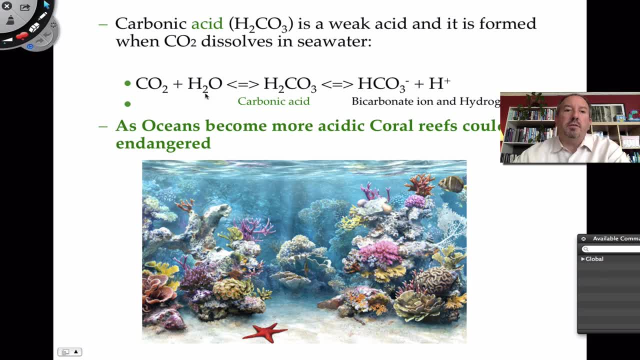 increasing the acidity of the ocean, And so here's the reaction, in case you're interested. in that It's: carbon dioxide in water produces carbonic acid. It's a weak acid, truthfully, But nevertheless. it then disassociates into bicarbonate ion and then H+, which is 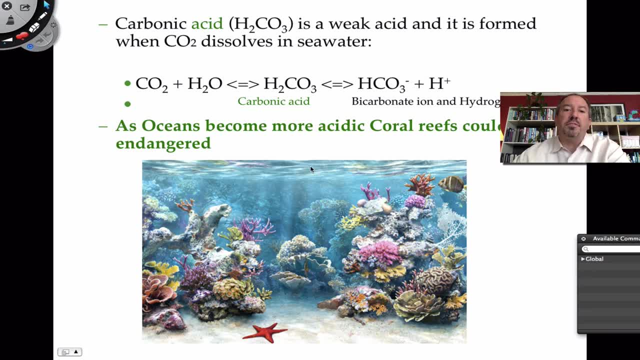 what increases the acidity, And so what happens is it's lowering the pH, And what's happening is: the most sensitive to this are the coral reef animals, And these coral reef animals. it interferes with their ability to absorb calcium from the water, and 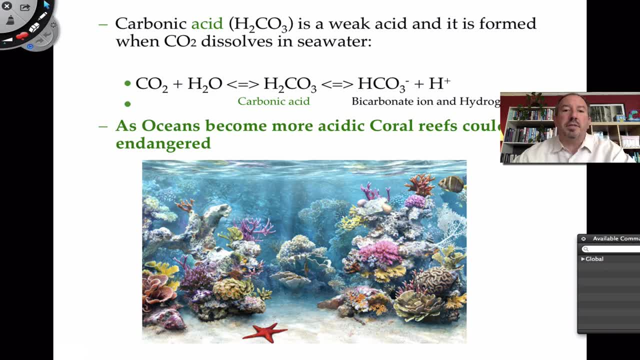 construct their shells which protect them, And so it's basically eroding. If you had, for example, if you were to do this at home, if you were to have, a piece of chalk which is a lot of calcium, try pouring some vinegar which is acetic acid. try pouring that onto the chalk. 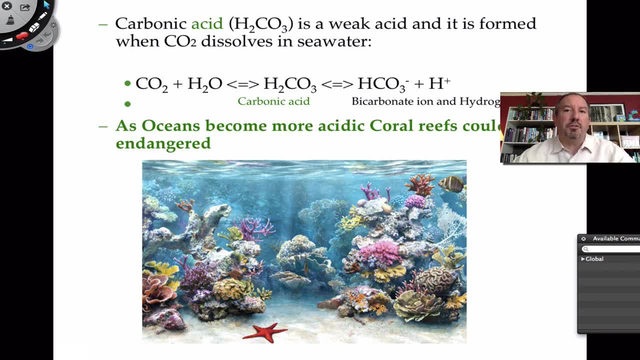 What it's going to do is dissolve it. And so that's what's happening to the coral reef: The acid is literally dissolving. And so that's what's happening to the coral reef: The acid is literally dissolving the coral reef. We can't have it. We can't have that happening, And so 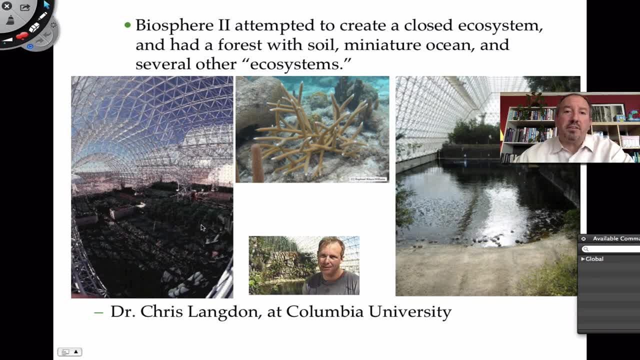 what's interesting is to determine the effects of this is inside the biosphere. They call it biosphere two because there was a biosphere one and then a biosphere two. So here's this ocean, And so there's a scientist studying this from Columbia University who's 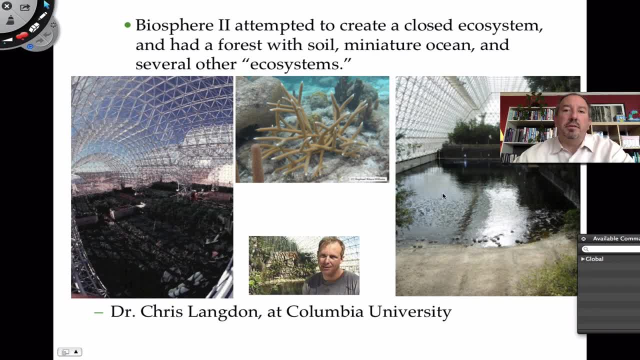 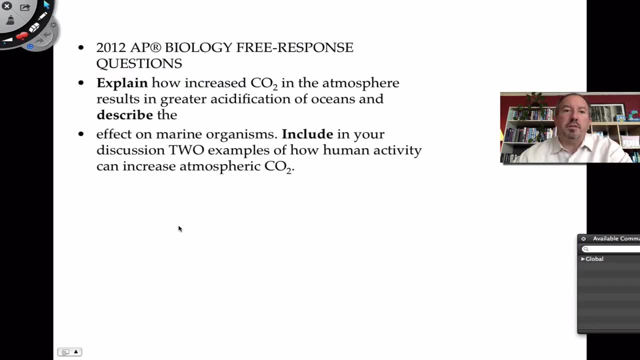 trying to analyze the effects of the acid that's occurring inside the ocean and how it's affecting the coral, And so that's kind of interesting. And then just to add a little relevance to this, you know and we have an advanced placement biology question coming at us, 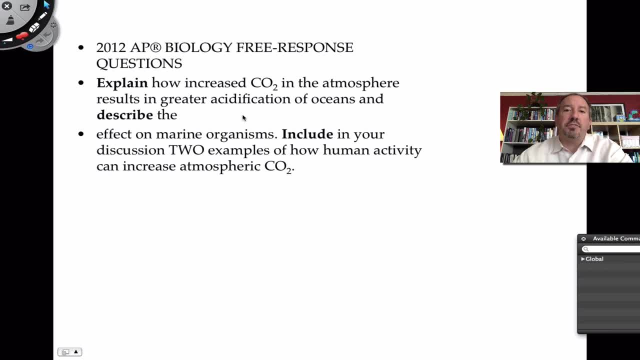 in the year 2012.. And it's literally asking. what we're talking about right now is how increased carbon dioxide in the atmosphere results in greater acidification of the ocean. So again, that's producing carbonic acid and then bicarbonate, And that's increasing the hydrogen ion and the effect in the marine organisms. Again it's. 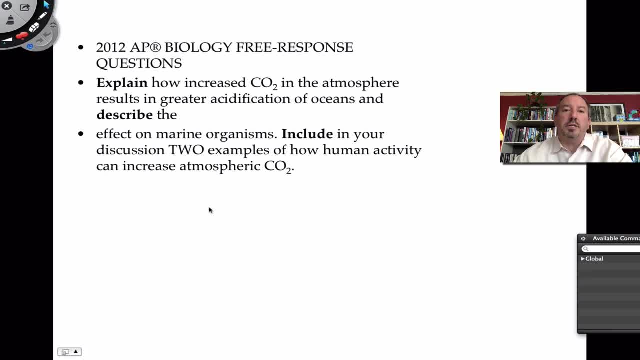 hurting the coral reef because we're not able to produce And so, as a result, human activity- how can? two examples of human activity that can increase carbon dioxide? And that's, of course, burning fossil fuels and combustion, And also the logging and deforestation is indirectly raising it. 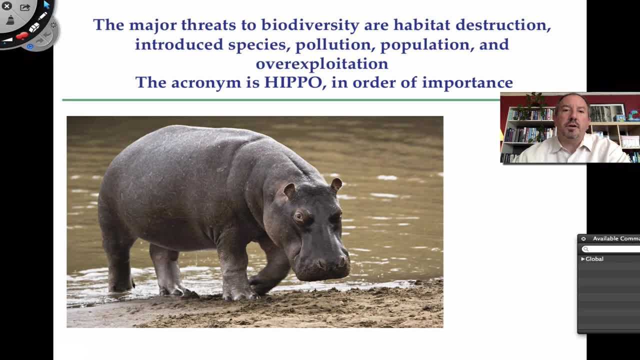 because the trees are the ones that are removing it, And so that's kind of interesting, And so I want to talk to you about the threats to biodiversity, And so you're like: well, what's going on with the HIPPO? To remember this, sometimes we need little acronyms to help us. 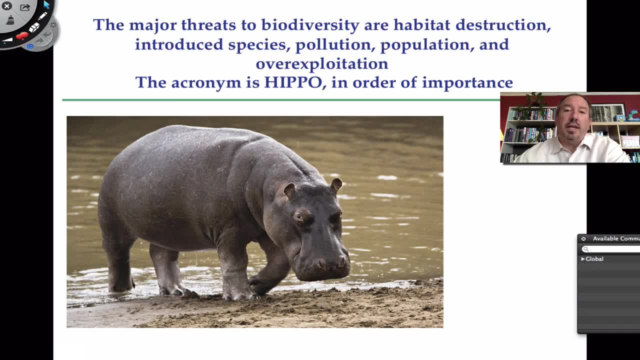 little memory hints to sort of remember things so we can carry this along with us forever. And so if you're going to get into a conversation about species, declining species diversity and you're like, hey, I recall they had something to do with HIPPO And HIPPO stands for you know, 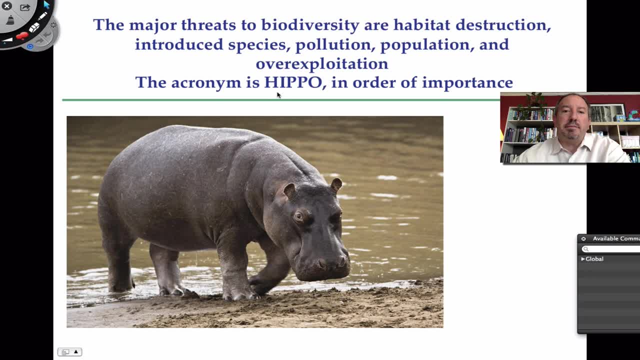 habitat destruction, which is the H habitat destruction, And then it's I for introduced species, P for pollution and another P for population. This would be human population, And then O would be overexploitation. And so this is a one way to remember this, And it's also kind. 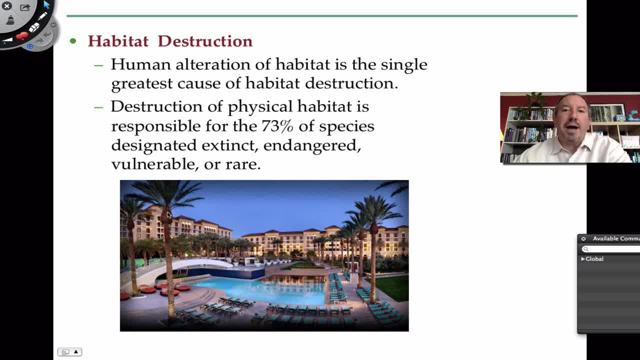 of in the order of importance as well, And so habitat destruction. I mean, this may seem obvious, but when humans alter the habitat- and I know we like, like places, like resorts, like, for example, in Las Vegas, and we create this, what's happening is we're removing the normal habitat that all of the 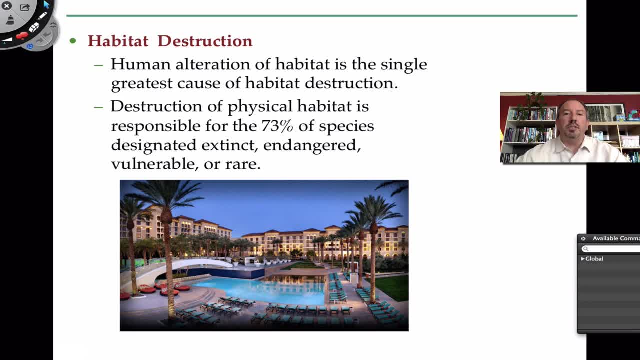 organisms are living in, And so when you do that, you lower the carrying capacity, and then organisms are going to be competing, And the loss of some organisms can affect the others as well, And so habitat destruction. it's: as we increase in numbers we take more of the world's habitat away, And so we we've even 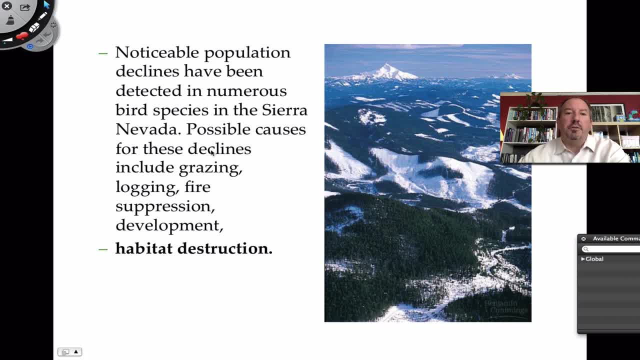 noticed, like for example in the Sierras, the Sierra Nevada, we've seen declines in all kinds of populations, in particularly in the birds. And why is that? Because they're of grazing land that we use And so that's a habitat destruction for logging of trees and also fire suppression. 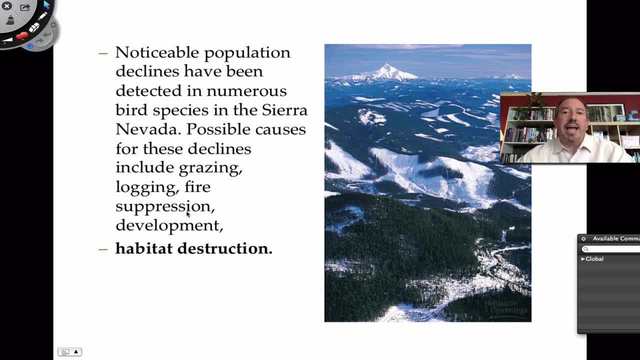 You're like, wait a minute. fire suppression? Yeah, Because that's habitat destruction, because ultimately it's not allowing that particular forest to be able to thrive in the future And therefore that affects the habitat And then just sheer development. as we expand and move outward, we're we're destroying the habitat, And so this. 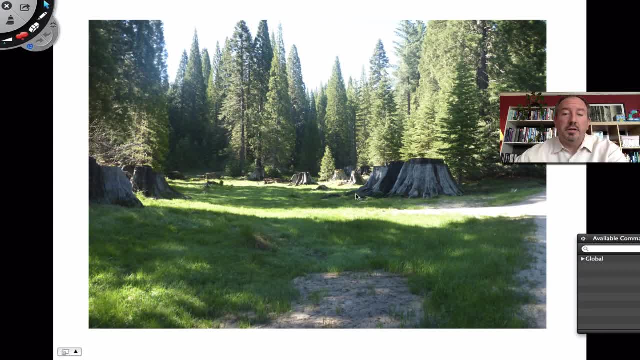 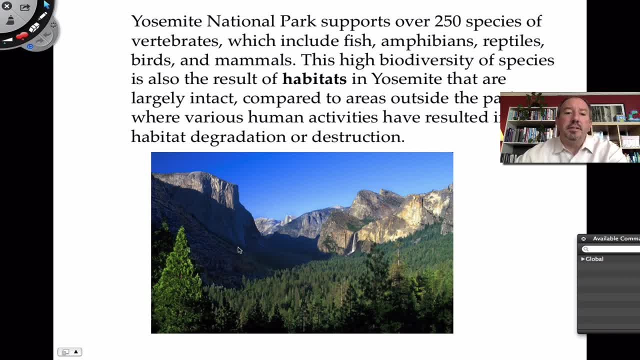 so we're fortunate that we have some areas that are fairly pristine. I say fairly, meaning that we have these beautiful parks like Yosemite National Park, And it's like: well, wow, look at all the species diversity there: 250 different species. 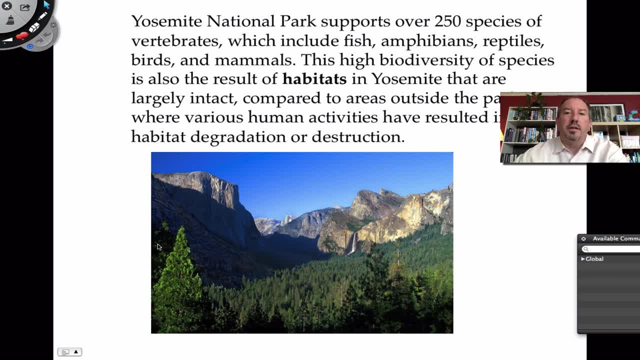 all sorts of things are living in there, And so it's sort of a really great triumph of biodiversity. And why? Because the habitat has been pretty much preserved. I mean, you can have a lot of trees that have been quite a long time. We don't have a lot of trees that. 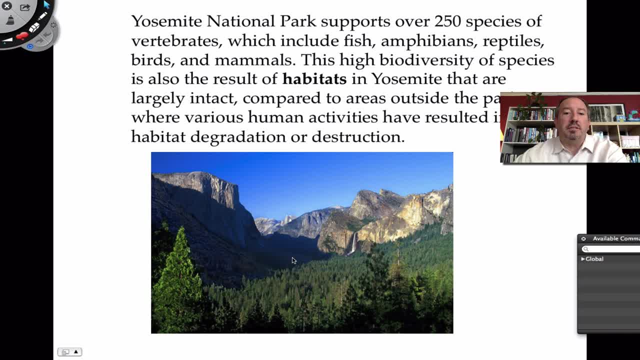 You could debate this in terms of the development that we see in Yosemite Valley, In terms of, also, the visitors that are coming are literally trampling the park to death. They're almost like loving it to death, But if you were to compare, it's still looking good. 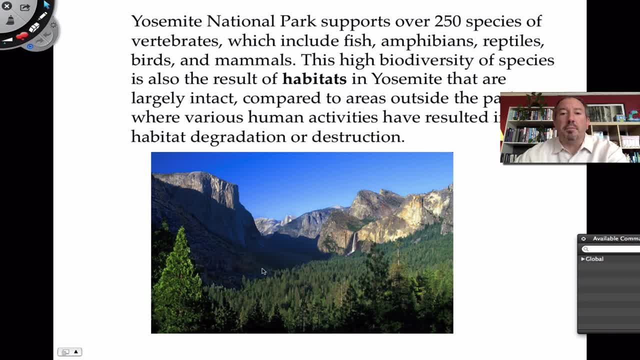 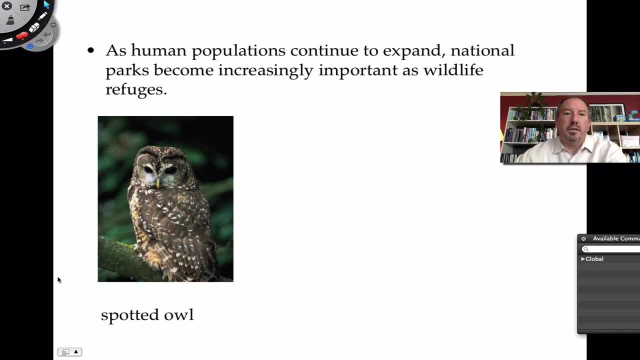 If you were to compare the species diversity within the park boundaries to just right outside, and there's a big contrast, and that's because of habitat destruction. And so an example of this is the fact that the spotted owl, so human population, continues to expand, but luckily the wildlife refuge in the national parks are saving these species. 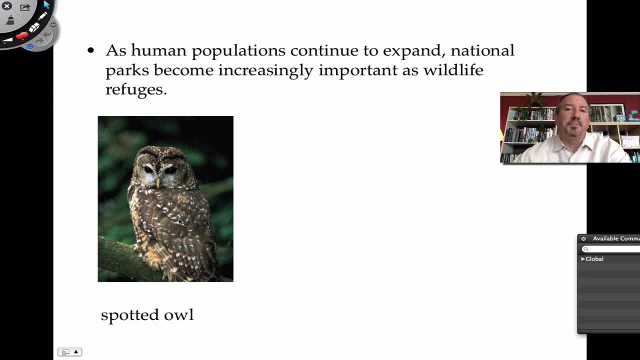 like the spotted owl. And again, the spotted owl gets a lot of attention and people scoff at it. Has anyone even seen a spotted owl Who cares? Well, again, it's a keystone species. I might bring that up again. 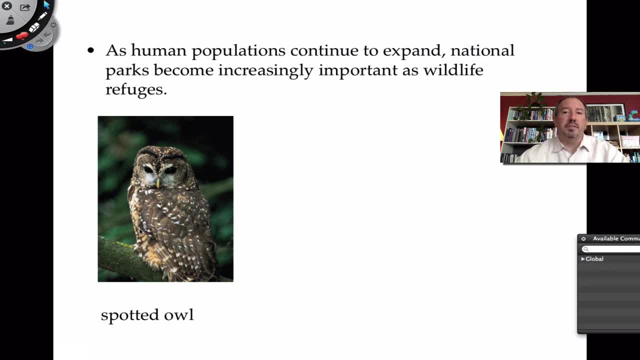 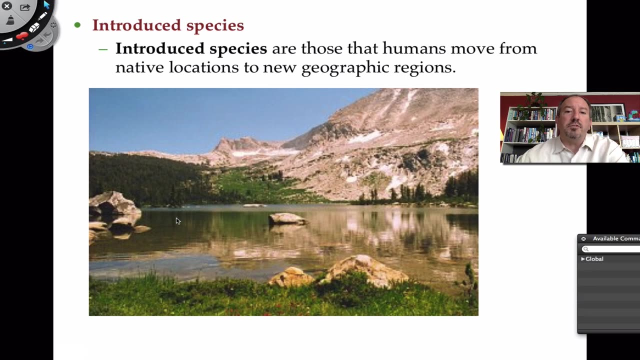 It's a predator, And so therefore, it maintains, Yeah, The balance in the food web, and it actually encourages species diversity. So it's not really trivial. And so next on the list is introduced species. Now, introduced species. there's so many examples of this. 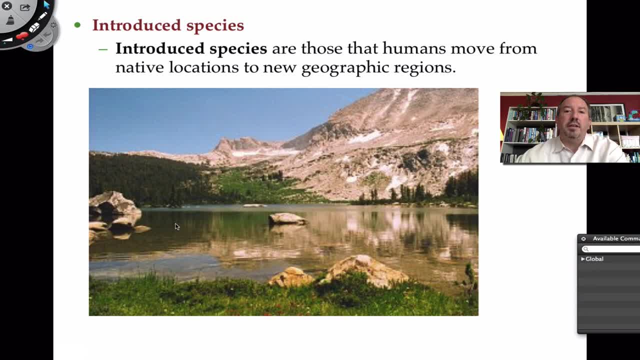 Even here in the Bay area, San Francisco Bay area- it's a place where there's lots of ships that come in, because it's a port where there's a lot of trade going on, And so these ships are also bringing in lots of introduced species. 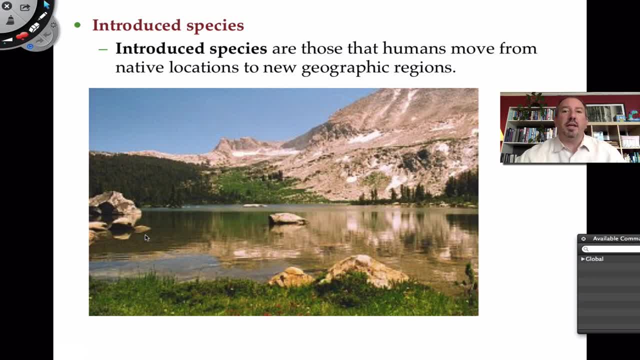 Indirectly, by taking in water from where they're, where they came, and then releasing that water when they come into San Francisco Bay. So there's all kinds of things coming into the Bay, which is reducing species diversity. But how do you like this example? 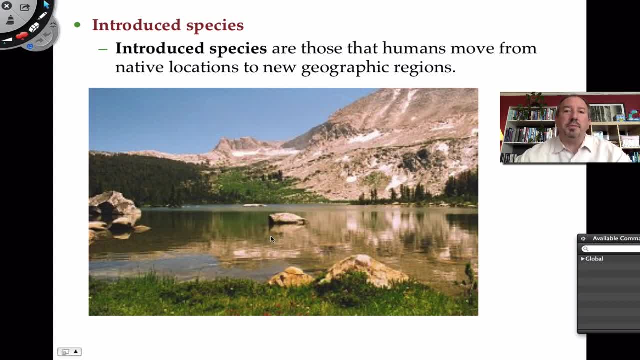 There's, would you believe. there was once upon a time in Yosemite. there wasn't a lot of visitors, And so to it was thought by the park service to increase visitation. people are into fishing, So they thought that they had actually. 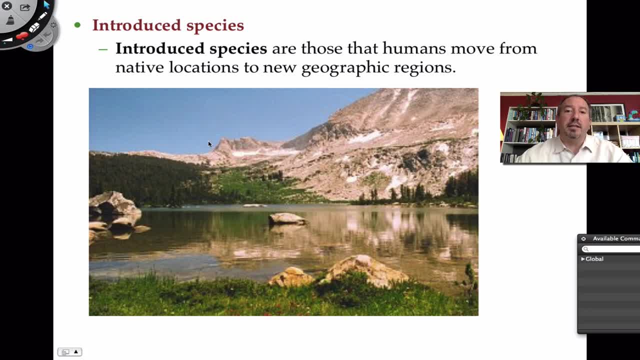 Fly over the mountain lakes, the high Sierra lakes, with helicopters and literally inoculate these lakes, drop in fish, And so they're. they introduced trout to these, to these lakes, and you're like, wow, that that'll be great. People love to come up there and fish. 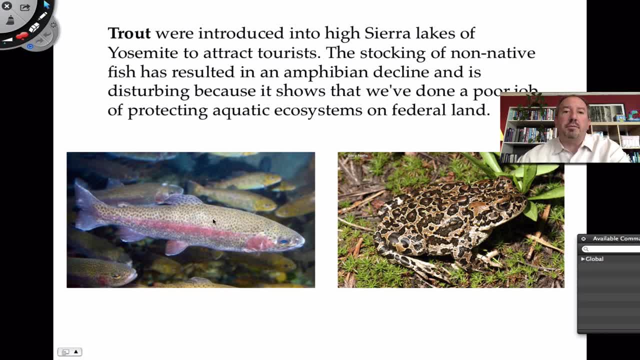 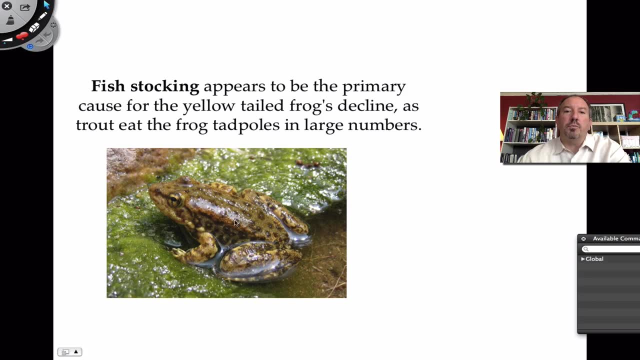 But as a consequences, it turns out, the trap that's up there, you know, may have been attractive to tourists, but what they're doing is they're eating the frog tadpoles, And so what we see is a dramatic Loss of of of native frogs that were once living in these lakes. 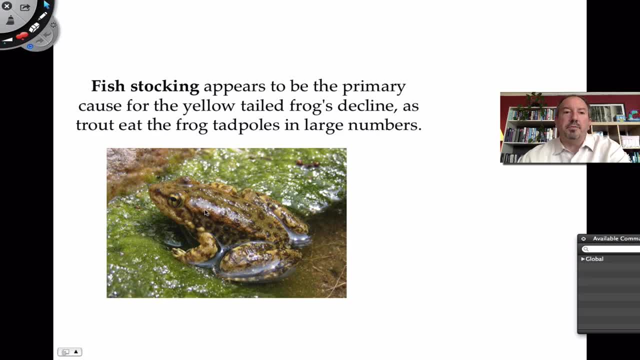 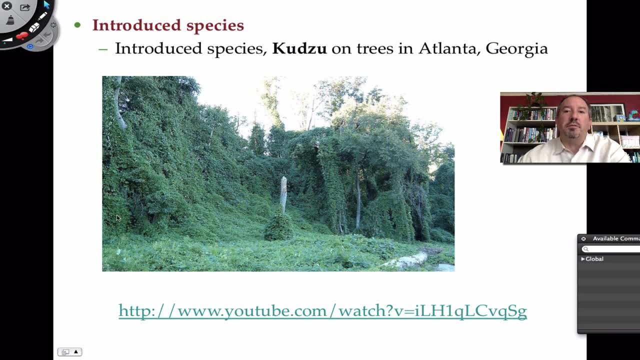 And so that's kind of a brutal um example of introduced species, One of the classics, classic introduced species. If you live in the South, you'd be able to identify this with this immediately. It's this plant that came from Japan called Katsu. 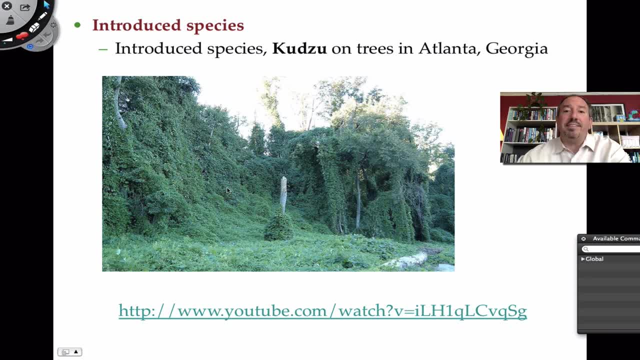 This Katsu is just growing like crazy. It grows really quickly And it outcompetes all the normal vegetation. It grows so fast that it's just literally like total weed. It grows all over the place, on the side of the road And it what it does is that it it's literally like choking out the natural vegetation, because 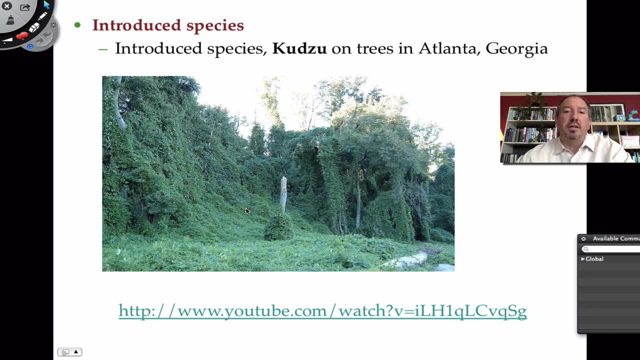 it's blocking the sunlight And so it just can't be stopped. It's like you can't cut it back, It'll grow. You can't poison it, Cause it'll it'll hurt other vegetation. It's just simply there's no natural predator for it. 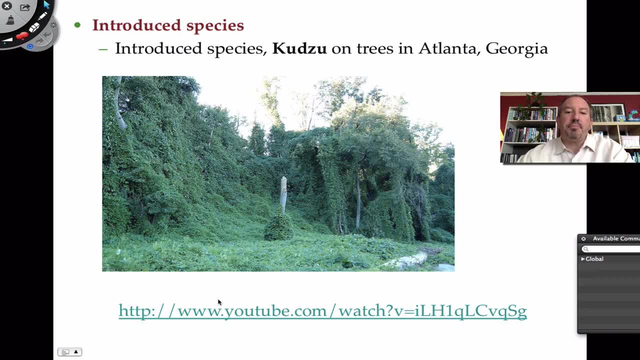 And so it's just out of hand. And so if you can see this link on YouTube, um, you're welcome to like grab that and take a look at the video. or literally, like type in Katsu and you could like watch this cool video on on uh Katsu. 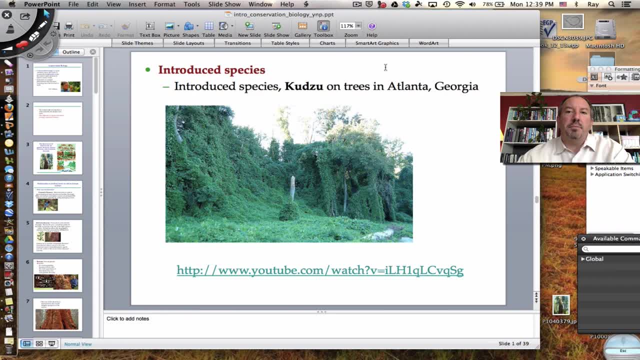 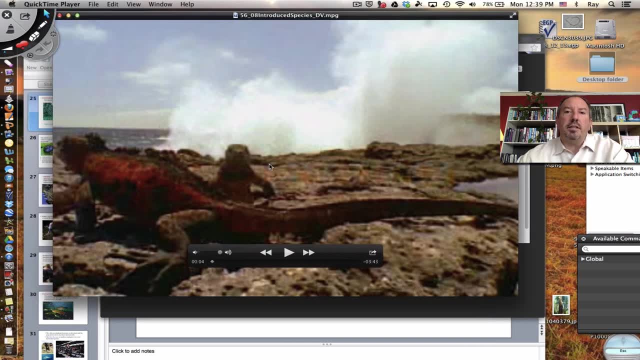 If you're really interested in that. I want to show you, though. um something that's kind of interesting related to uh introduce species is um on the Galapagos islands. you know people think of the Galapagos islands a lot. 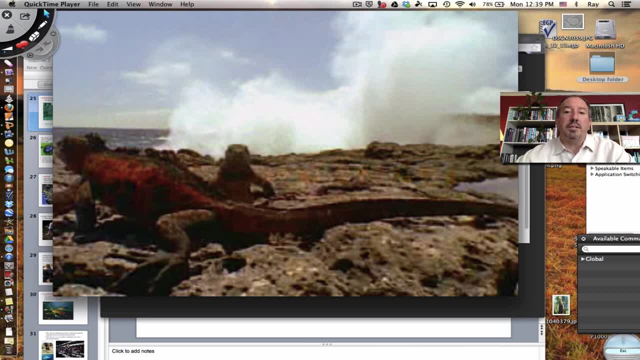 Okay, We think of Charles Darwin and the theory of natural selection. We think that these islands are, are just out there and they're and they're very remote. They are, but there's a tremendous amount of tourism on the Galapagos islands and there's 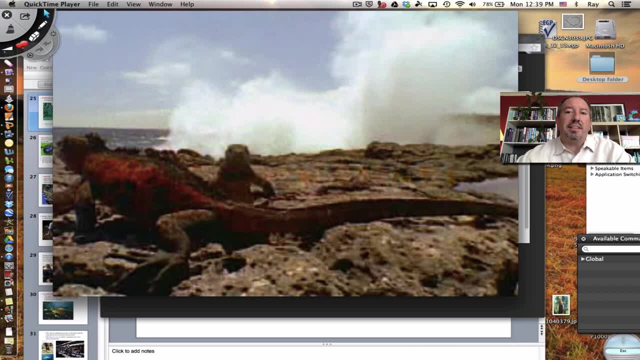 actually people living on the Galapagos islands And, sadly again, the tourism and all the people that have that that arrive on the Galapagos. they're bringing a species that don't belong And so they're introducing them. 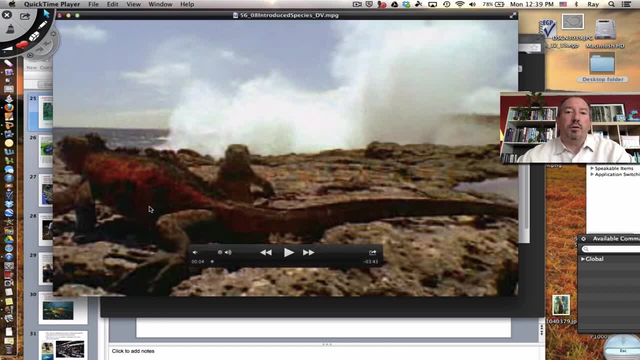 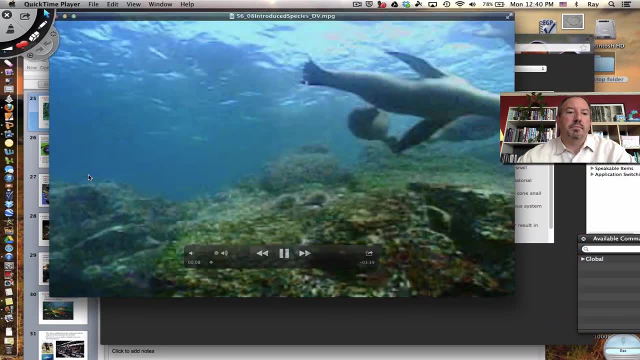 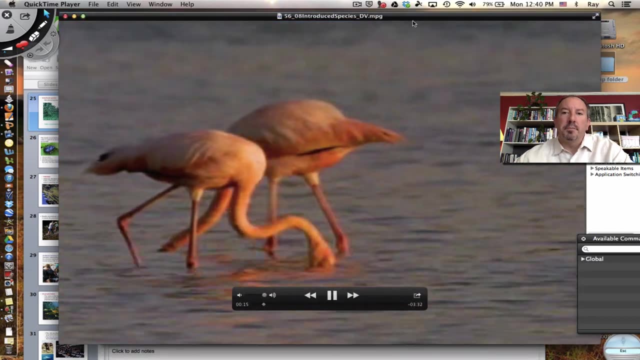 And these species are are threatening The organisms that live there. Take a look at this video. I think you'll enjoy it. The islands of Galapagos, located about 600 miles west of Ecuador, are famous for their unspoiled beauty and unusual animal life. 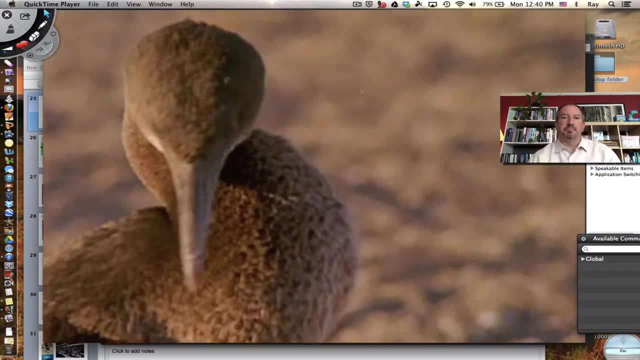 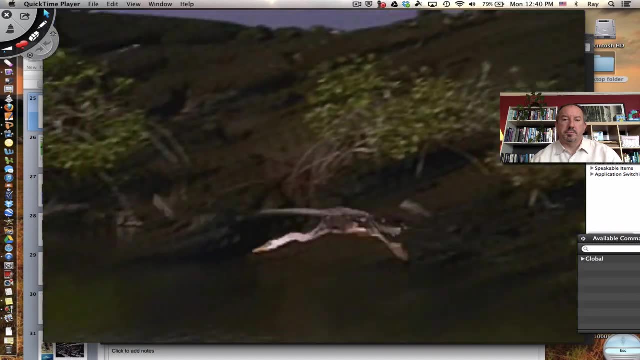 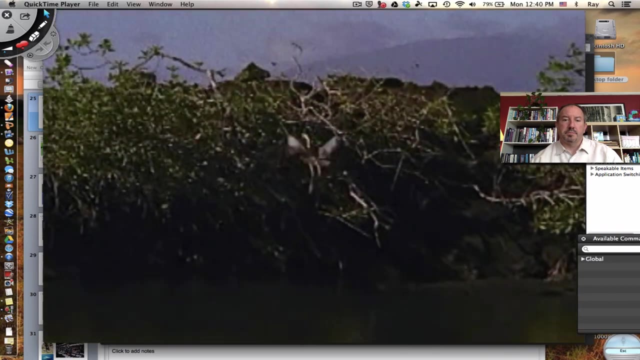 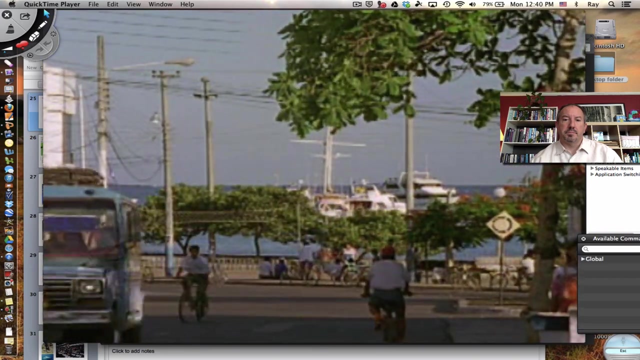 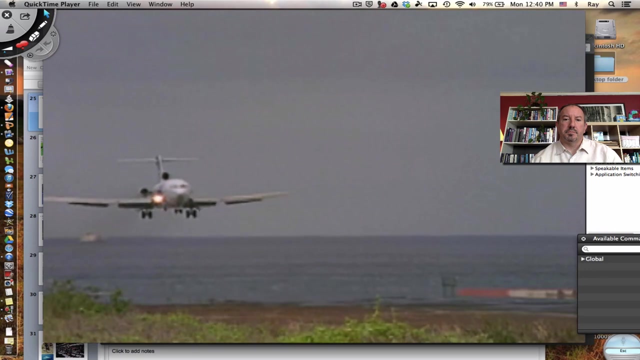 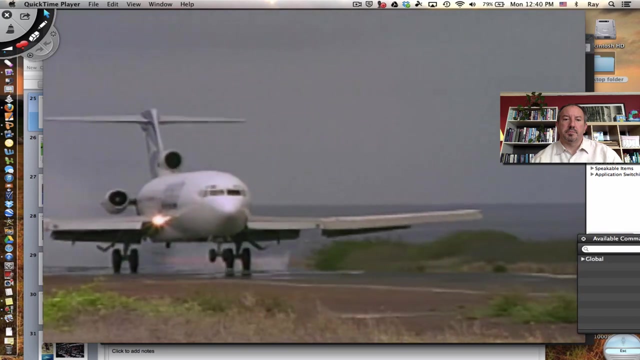 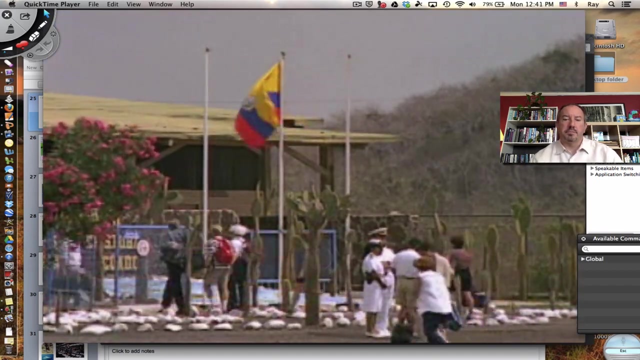 Creatures like giant tortoises, flightless cormorants and swimming Marine iguanas evolved in relative isolation here. Okay, Okay, Okay, But these conditions have changed dramatically on several islands of Galapagos in recent years. natural state they also introduce other items that harm its fragile ecology. 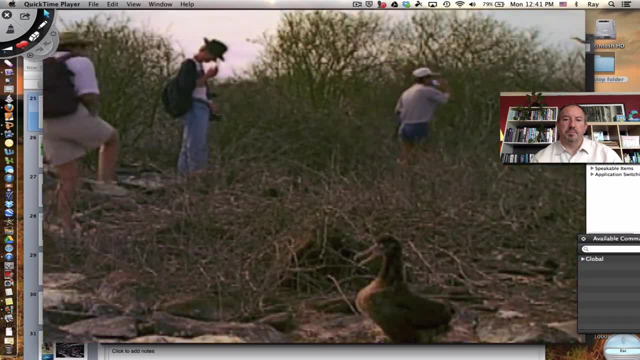 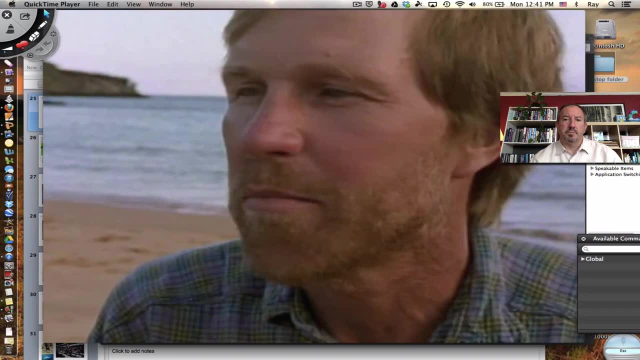 Paleontologist, Dr David Stedman, explains. Even in a place seemingly as remote as Galapagos, I mean, there are more than 50,000 tourists a year coming out here. So the beach we're sitting on, boy, what a wonderful beach. It looks great And within a 50-foot radius of us. here you know. 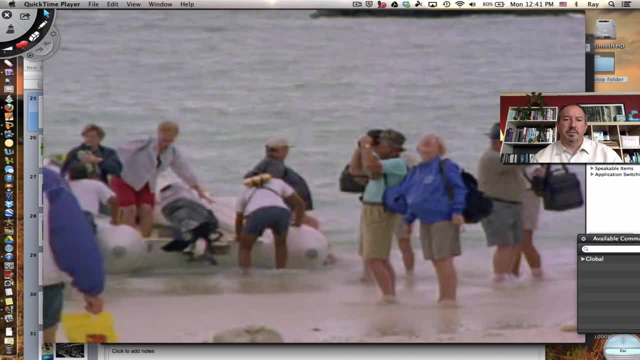 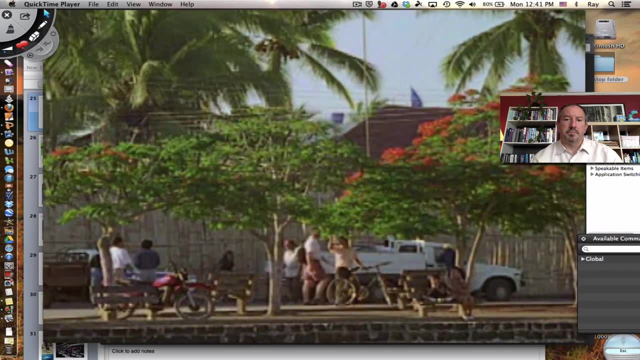 you can pick up a thousand pieces of garbage Now. garbage in itself maybe doesn't cause extinction, but nevertheless it represents a type of human impact. Today, the biggest threat to native populations come from introduced species: Dogs and cats, farm animals and rats. 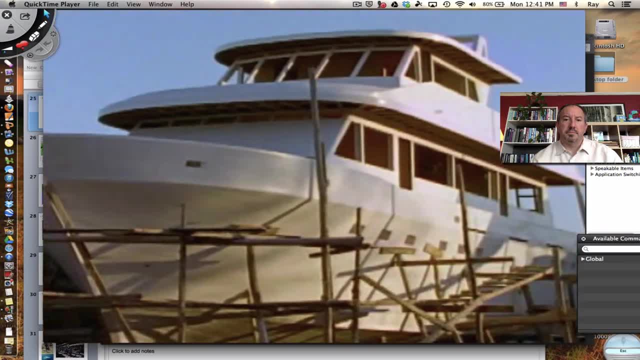 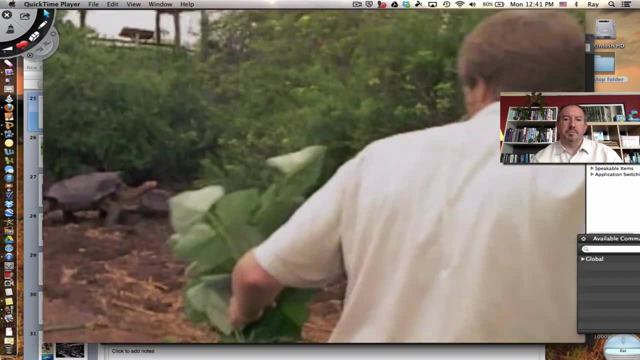 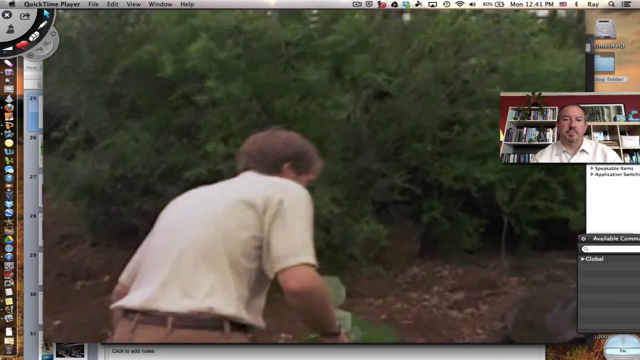 arrived on ships over the years. When they get on islands, they're just cut loose. There's virtually no check on their populations, So their numbers grow rapidly and they have devastating effects on the vegetation. They also have a devastating effect on animal populations. 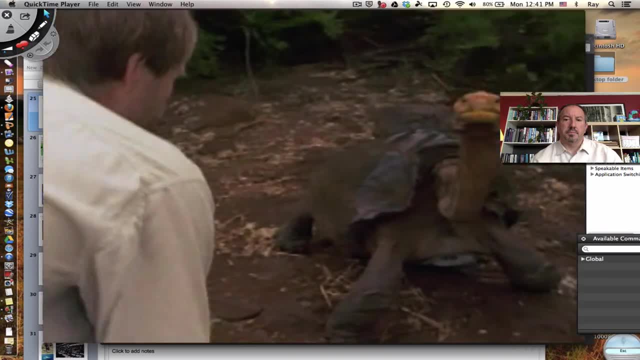 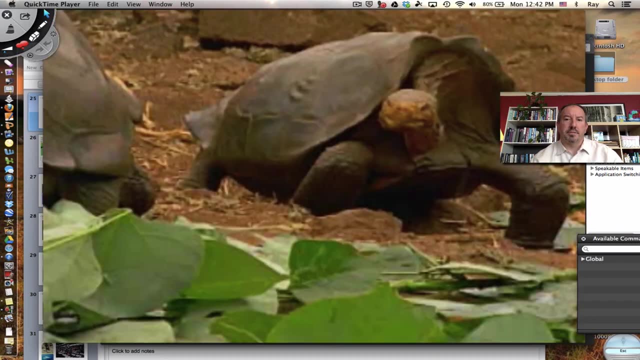 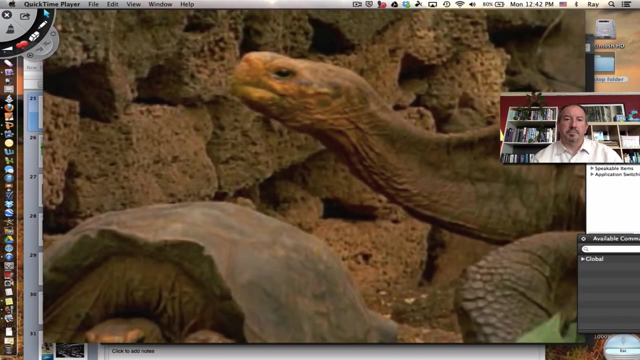 One population especially threatened is the giant tortoise. In an effort to protect them, wardens from the National Park dig up their eggs as soon as they are laid and bring them to the Charles Darwin Station. Here they are supervised and kept out of harm's way. 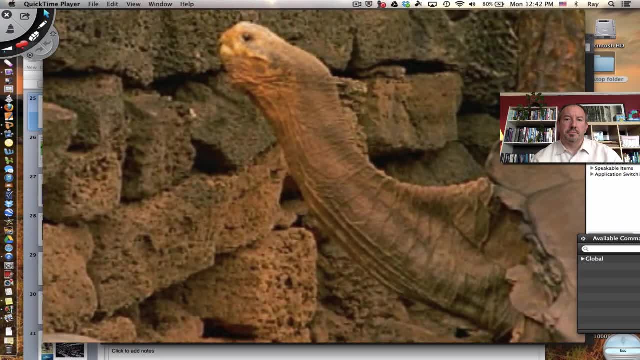 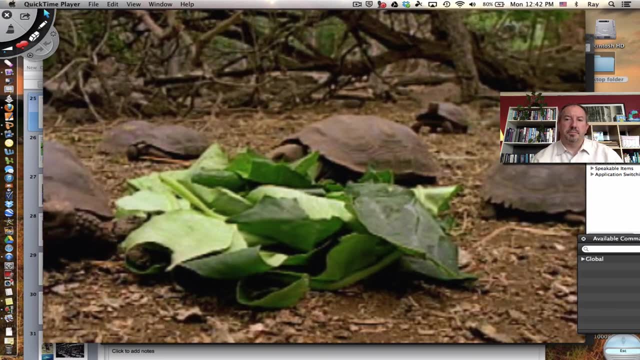 until the tortoises are big enough to survive on their own. These are three-year-old tortoises from the island of Santiago. Santiago is an island that has a lot of problems with introduced species, and so, even though there's a wild population of tortoises there, 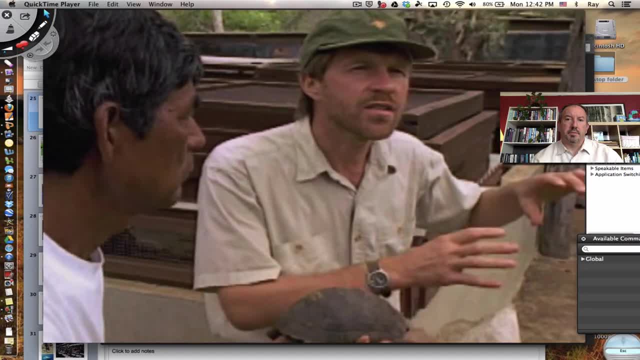 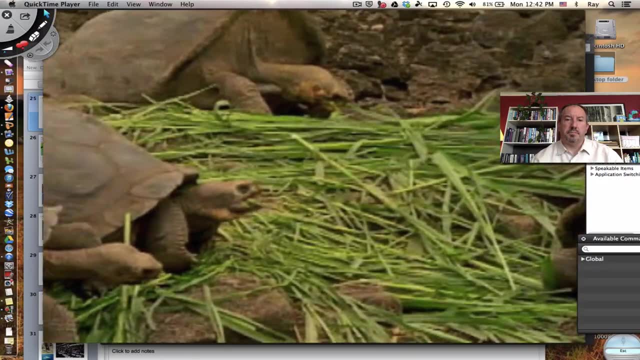 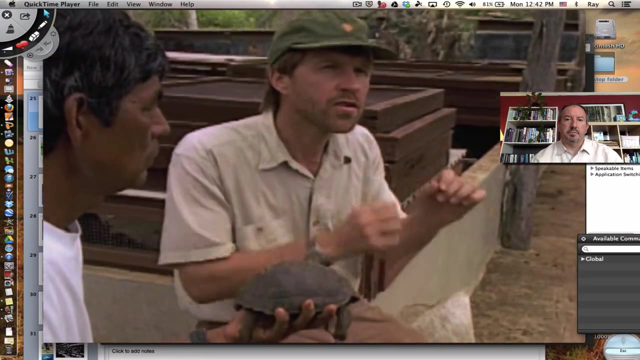 that in fact can lay eggs in the wild. the eggs are eaten, especially by rats and pigs. Once the tortoises hatch, they're raised here until they are four or five years old. By one year old these tortoises are sort of rat-proof. so a rat can't hurt a tortoise. 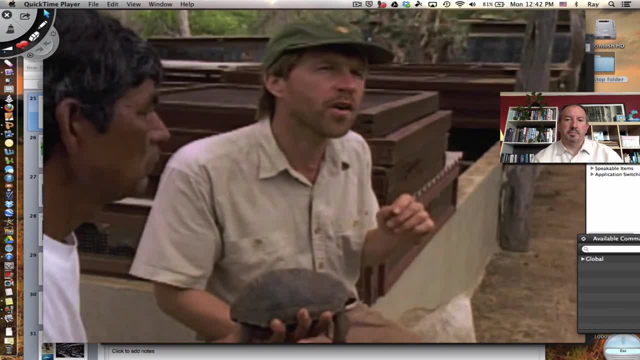 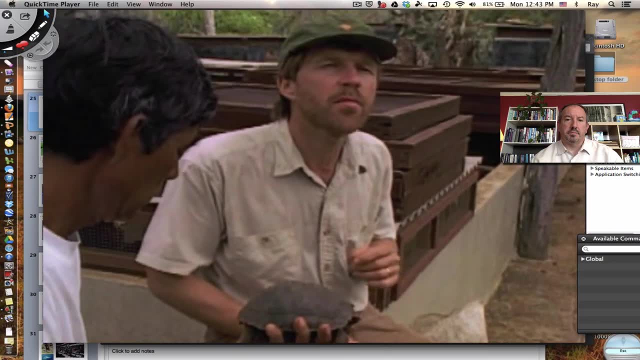 after it's about a year old, But on Santiago, with all the feral pigs they have. they have thousands of feral pigs on Santiago. The tortoises- these poor little baby tortoises need to be about four or five years old before they're pig-proof. So this is a good example of very 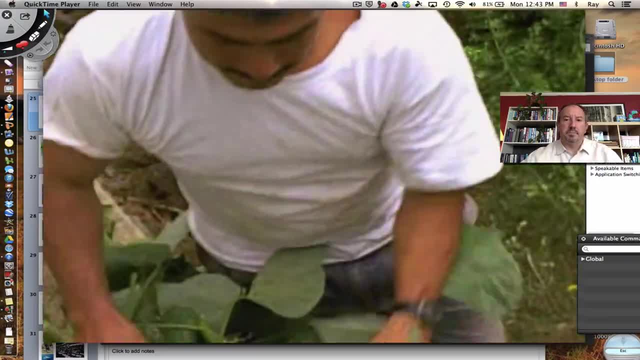 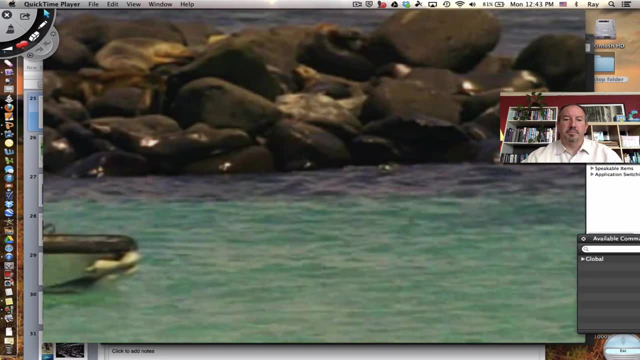 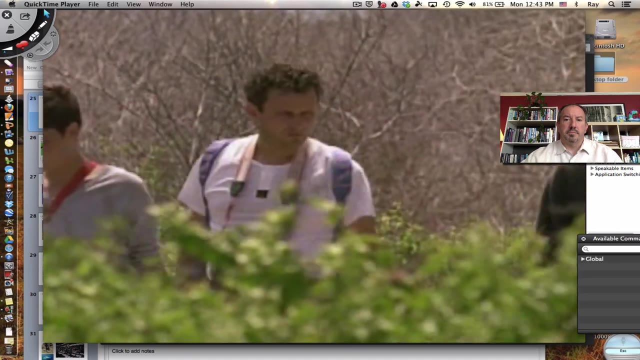 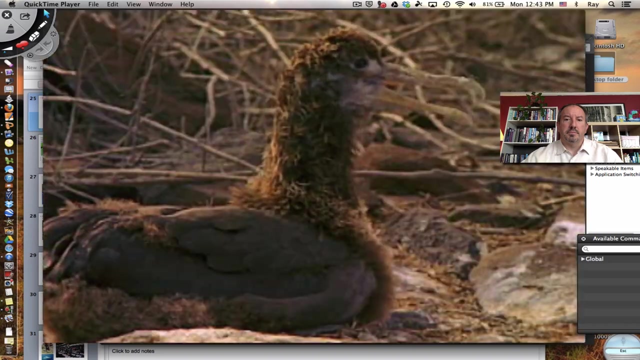 active, hands-on manipulation of a wild population in order to keep it going. When new organisms are introduced into an existing ecosystem, they create different, sometimes harmful, links in the food web. Often with added competition, native species cannot survive. Scientists like David Stedman monitor places that are changing in an effort to influence the chain. 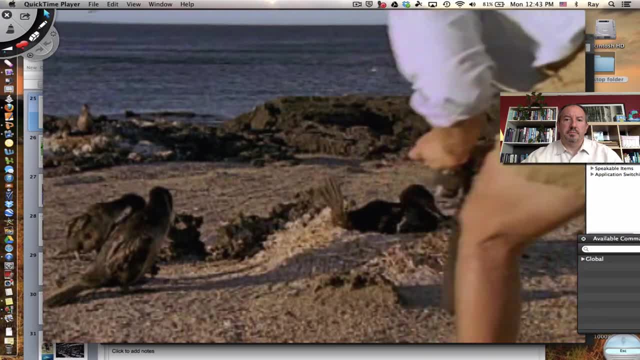 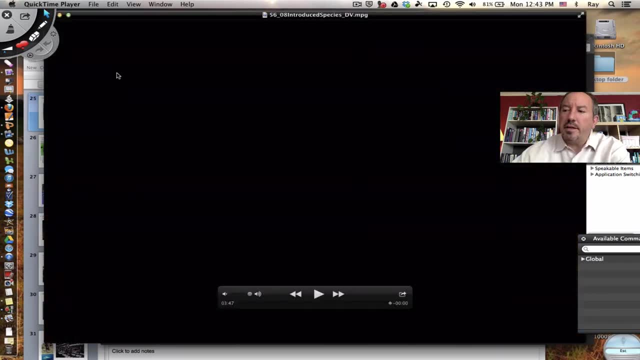 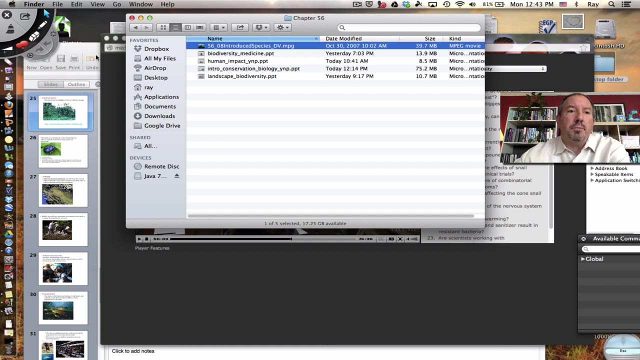 of events and protect the natural environment. So I hope you enjoyed that. The message that I get from that is: you know there's a couple of ways that you could go about steadily improving your environment and the environment itself, But when you get to the point where you're really focused on the environment itself, 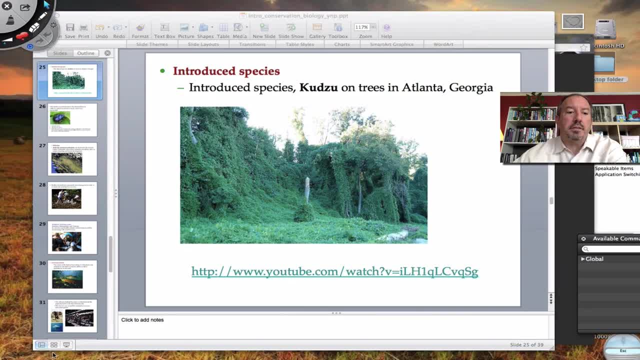 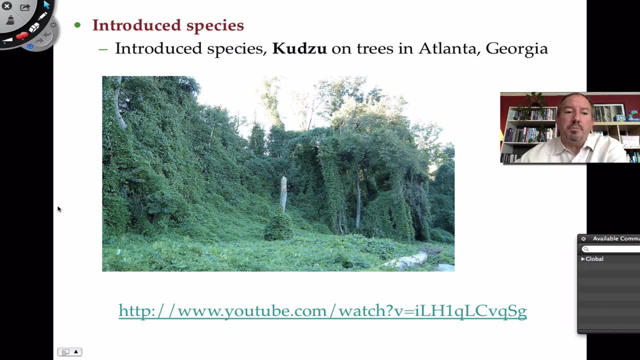 studying this. i mean, one thing is awareness to the fact that introduced species are an issue, but you could study them like a scientist would study them, and i'm hoping that you'd be interested in that. but you can also volunteer. you can go to galapagos islands and you can actually protect. 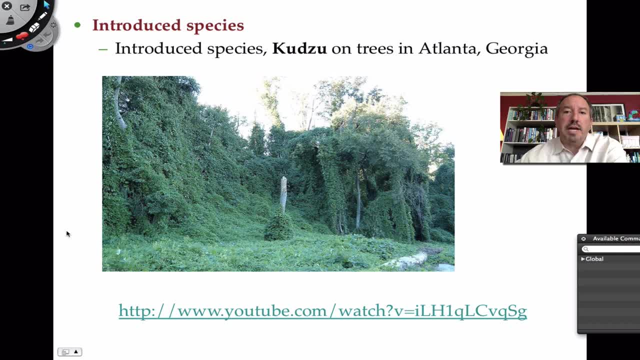 those eggs by working in those nurseries to protect them from those rats and pigs and dogs. but you're like, well, i don't know if i want to go to the galapagos islands or something like this, but again you could do that, locally investigate it. this is, it's a call. it's a calling we've got. 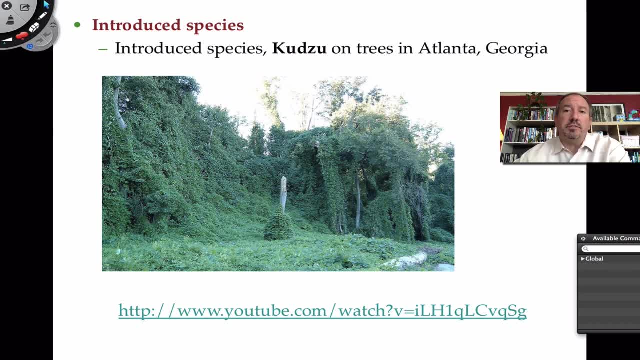 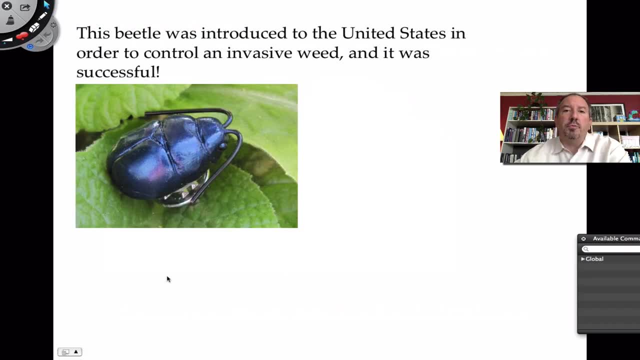 to step it up, like what's happening locally in terms of invasive introduced species and what can we do to protect the local habitat from this. and so one example of what can be done is we were noticing that there's this invasive weed that was grown in california by the klamath river. 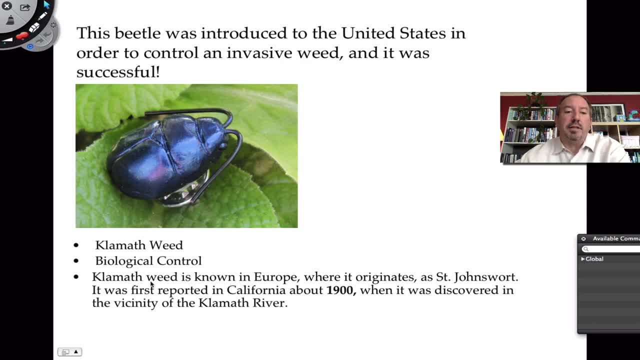 and it and uh it's. it came to be known as the klamath weed, but really its origin is from europe, and it was known as saint john's wort, and again, it was grown out of control, and so there was nothing that was keeping it in check, and so what we had to do is 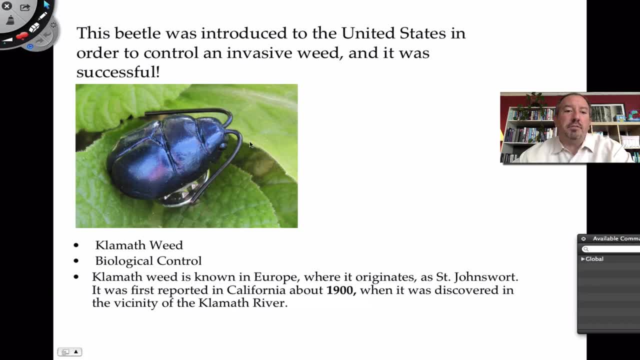 scientists from the university of california, davis like, researched this and they discovered that there was this beetle that sort of eats it, and so we went and got that beetle and started putting it into the klamath weed as a biological control. and so how do you like? 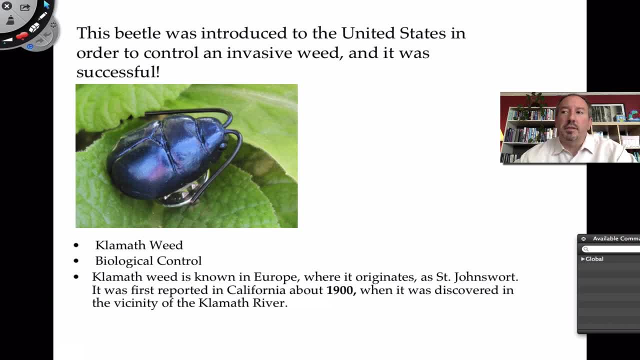 it. it's sort of fighting fire with fire, and you might think that there's some- you know- concern about this, when you're introducing something and it's causing a problem and then you're introducing something else in order to control it, and that, could you know, that can get out of hand too. when you're trying to manage nature, uh, it's more difficult. 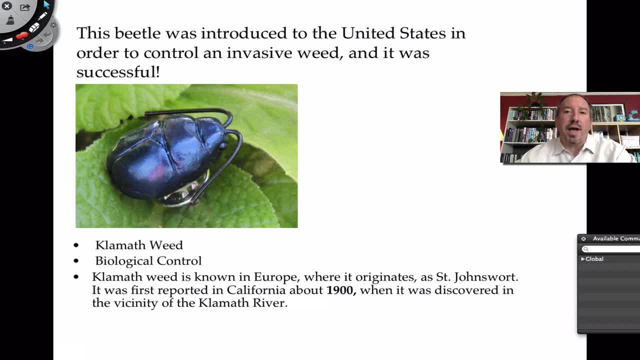 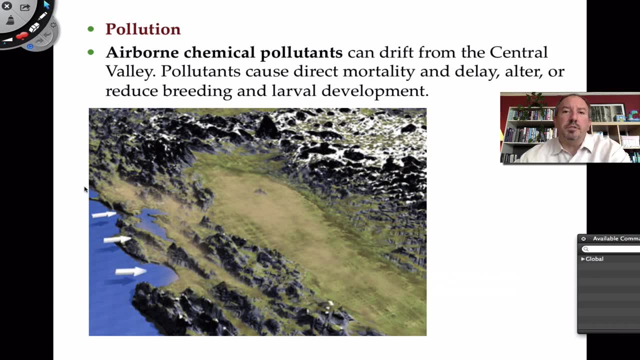 than it sounds, but i just wanted to point that out- that one way to combat this is to fight. fight it with another introduced predator. so another concern is pollution and again that we were watching just a second ago introduced the fact that tourists sometimes bring pollution and and uh things to the, to the habitat which hurt it, but more more often than not it's like for 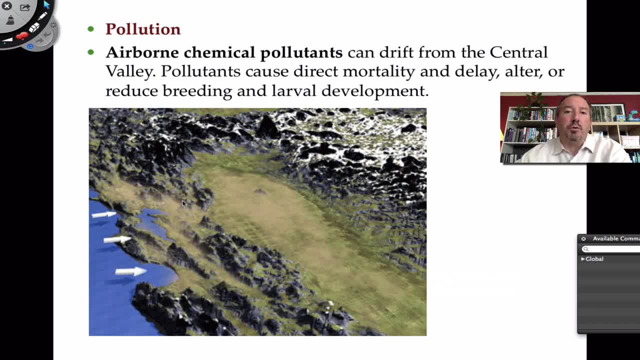 factories produce a lot of pollution, and so factories like oral refineries and such in industry produce some sulfur dioxides and nitrous nitrogen, containing compounds that can produce sulfuric acid and nitric acid, and it can cause acid precipitation. but sometimes the this airborne pollution, these chemicals you're like, well, it's only going to hurt. 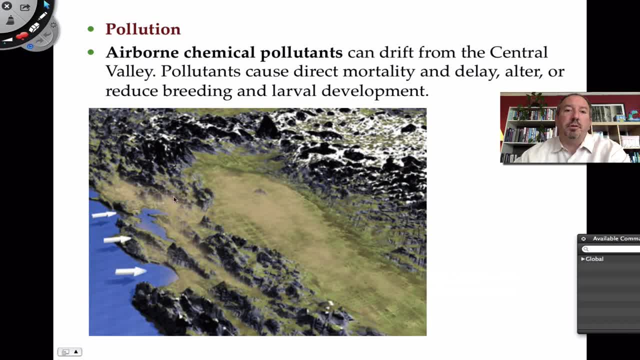 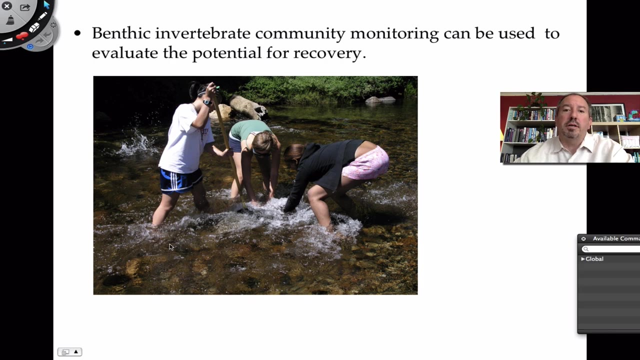 it locally. but no, when there's winds, that blow can blow these pollution pollutants across the central valley and they actually will hit the western slope of the sierra and and, as a result, will actually run down in the water when it rains, and so it actually enters into our most pristine environments. sequoia national park- yosemite. 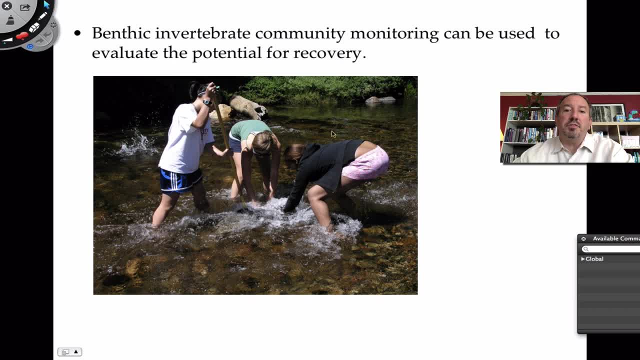 national park, and so would you believe that the tuolumne river, which is the main source of of water for the bay area, the tuolumne river, in merced river or the, the acidity is increasing as a result of this of pollution, and so you could monitor this. by checking this, you can check the ph. 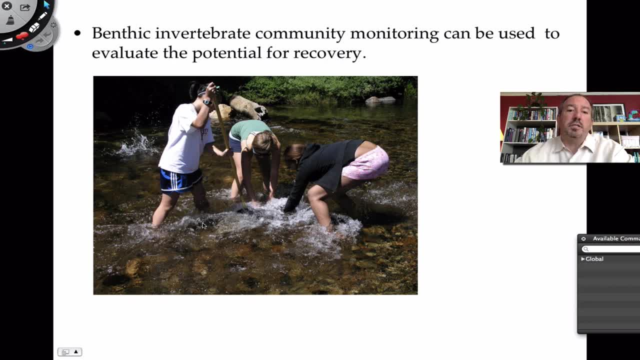 but you could also see what the effects are in the organisms that are living there. so at the base of the food chain, what these students are doing is they're picking up these rocks and then rubbing their hands on them, and then this student has a net and they're collecting them. these are called. 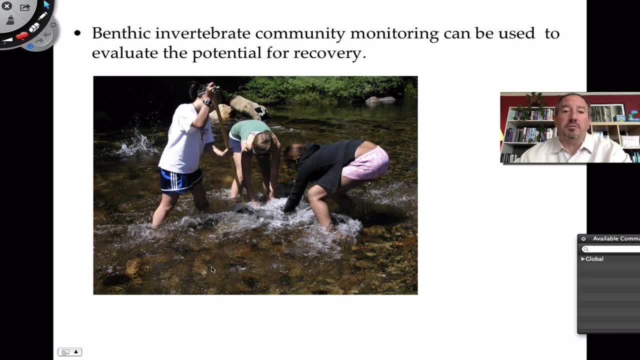 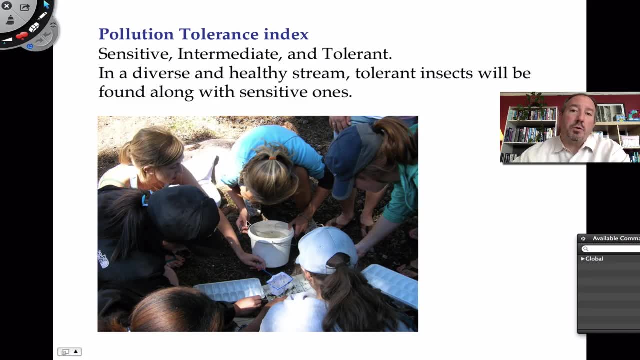 macro invertebrates which are- it's a little funny because they're really small little bugs and larva. and so what happens is some of these organisms are more or less sensitive to the to pollutants, and if you, by determining and counting those populations, you can determine just how well the 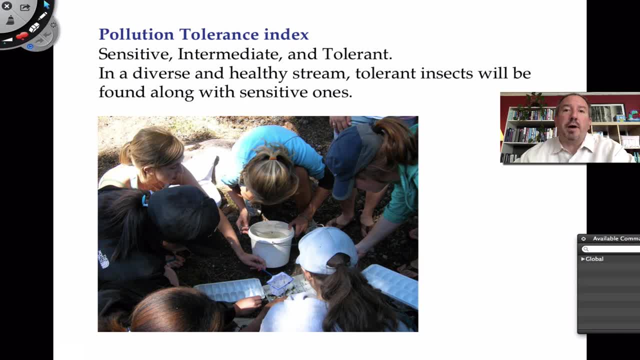 river is doing. it's sort of called bio monitoring, bio stream monitoring. it's very interesting and you can sort of determine and you're like, well, who cares about the bugs? well, the fish eat the bugs, and then the fish, and so it's really talking about the whole measure of the quality of the river. 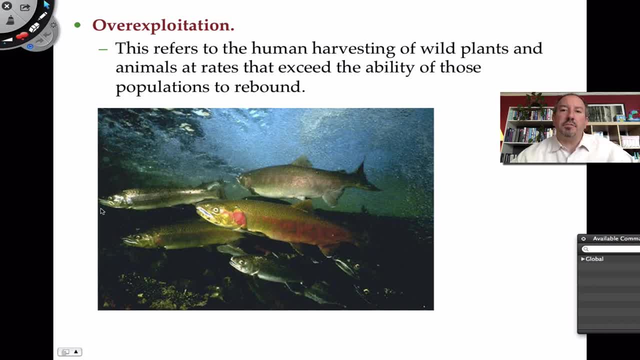 this is kind of sad too. again, all of these- i hope you're looking at this in terms of human- is causing this, and so over exploitation. we have a tendency to over harvest things that we really like, and, of course, salmon is a classic example of that that we've start devastated these salmon. 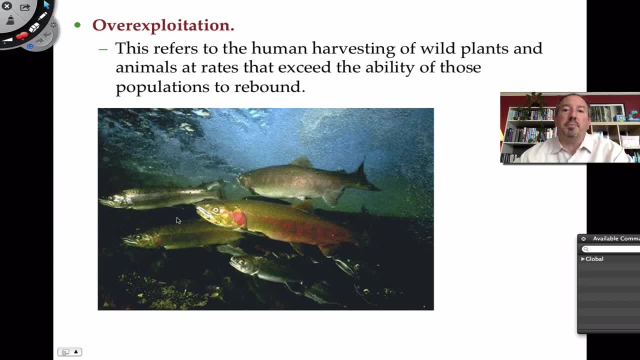 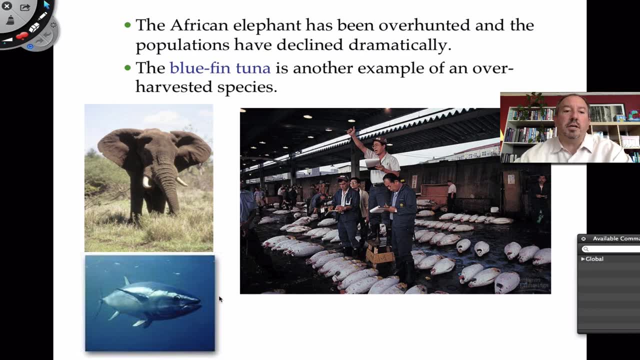 fisheries as well as other major fisheries. again, this is a topic that would come up in environmental science and in marine biology. but some examples is that this blue fin tuna. i mean we just love it. but we love, loved it to a point where we've over harvested. 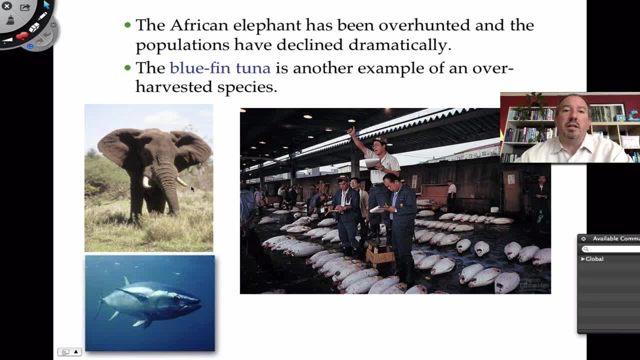 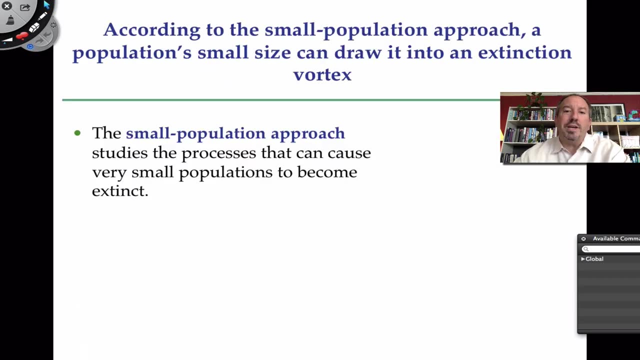 and it's endangered now And then things like the African elephant: so brutal- You can tell it's an African elephant because its ears are shaped like Africa. But we're murdering these elephants for their tusks, for the ivory. It's unthinkable. And so what happens is: you're like. 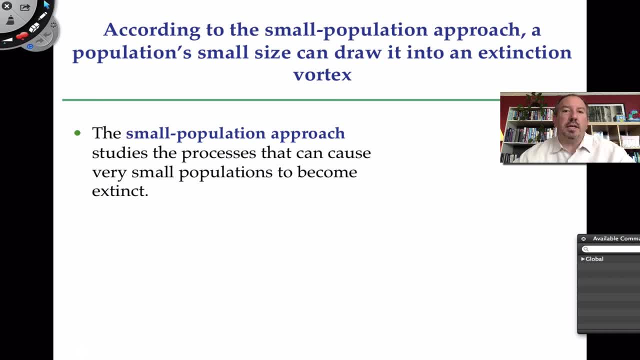 well, we'll just stop. We'll stop hurting the elephant and the population will come back, or the tuna will come back. Don't worry about it too much. Here's the problem: When the population becomes very, very small, what happens? Studies have shown that when a population is very small, 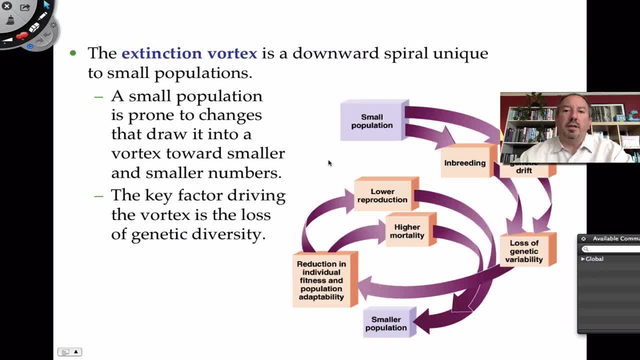 they start to inbreed with one another, And when the inbreeding could possibly lead to recessive traits manifesting, And then, as a result of that, you lose genetic variability and you get the same organisms Breeding with family members, And so there's higher incidence of troubled genes appearing in. 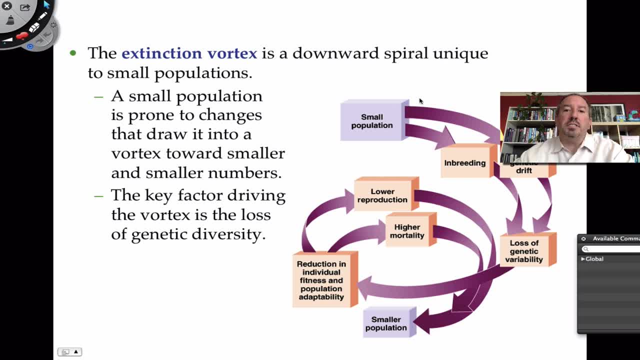 the gene pool, And then again, when a population is cut down by hunting. you're not cutting the population down and saving only the best, the most adapted organism. You're randomly destroying the population, And so what you can get is just a small group of pitiful. you know, just saying. 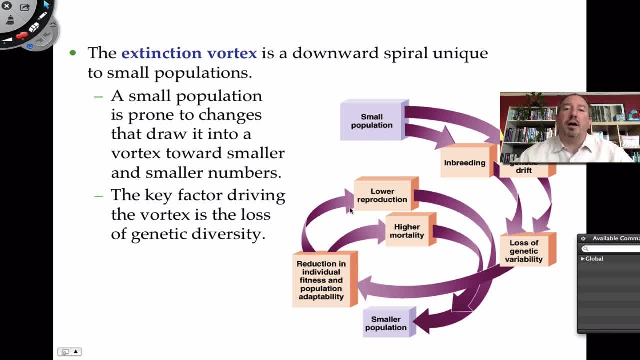 organisms That, when they're bred back up, lead to trouble, And so the population tends to have a higher mortality rate because maybe it's not looking good, which then leads to lower reproduction, which then causes a decline in the population, And so what conservation biologists call this is. 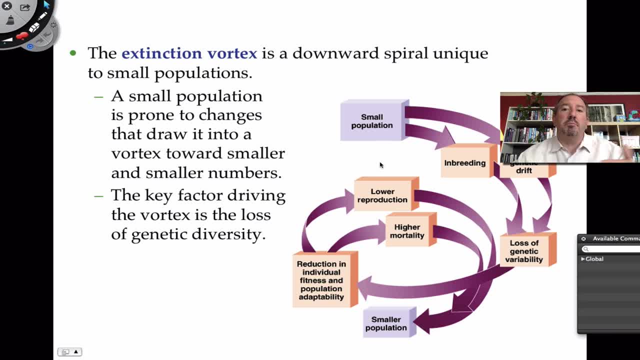 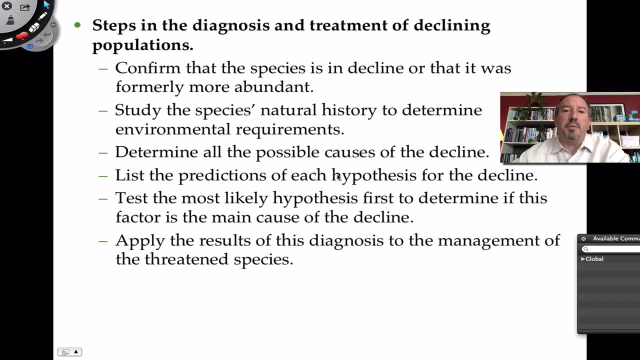 an extinction vortex. Once the population number gets down low enough, it's not going to be able to come back because of the loss of genetic diversity. Steve, check for landing sites. Everything is about display, And so that is what we variants are called. So we do that. using our tracks data, we can baggage out official. 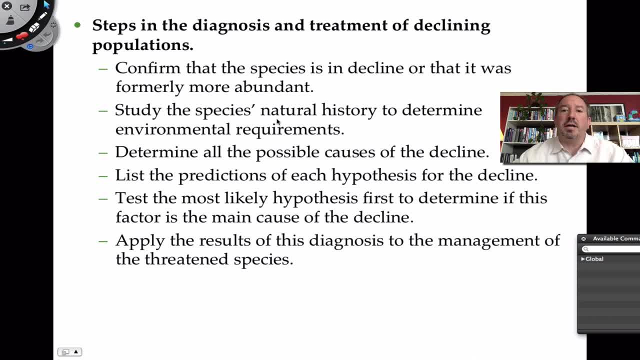 details, forヒ doesn't piping, but the data for the biological organisms that are currently stored in the healthy small group. You have all those hits When the ANC list starts to to go down, and so we start to years ago, when competition it's the alpha boy. irgend spielt years ago. like: So what are we going to do about it? So when you're concerned about a population that's declining, you have to take a systematic approach, as this is a science. I just have to confirm that the species in decline was once formally abundant. 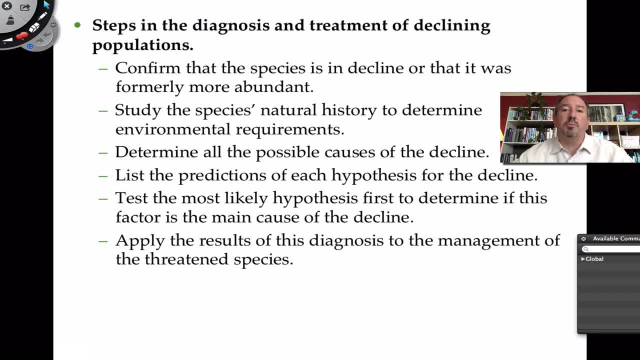 how many females? what are its special environmental requirements? It takes a long time to study this. And so what are the possible reasons for decline? Is it habitat destruction? Is it introduced species? And then you come up with a hypothesis. Well, what can we do? 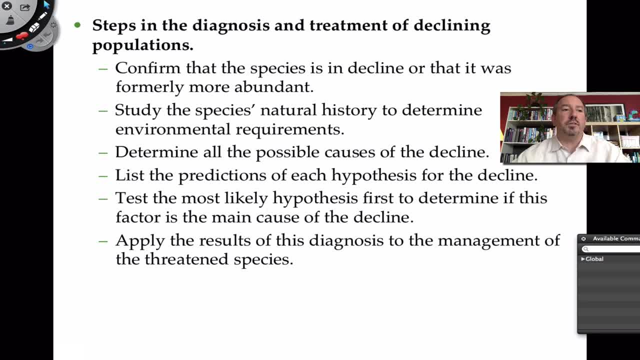 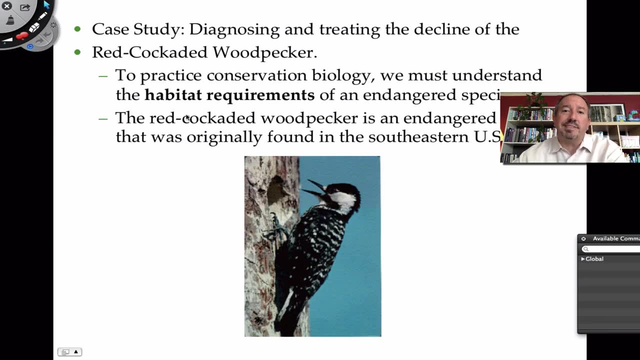 If we restore this, if we stop this, if we do this, then if, then what would happen? And then you have to go out and try it, And then, if something's working, then maybe a new management policy comes into play, And so an example of this is this. it's a classic In the southwest: 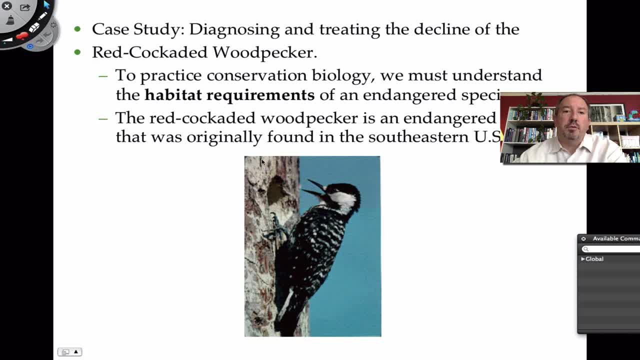 United States there's this woodpecker called the red-cockered woodpecker, And so it was once really, really, really prominent because of the forests that were once in the south. But a lot of that has been cut back. now It's been reduced- almost all of it actually- And so it's on the 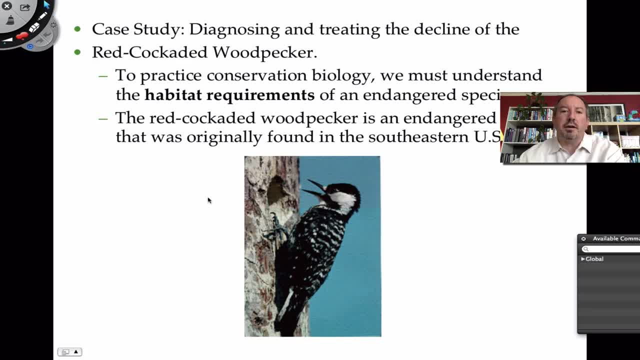 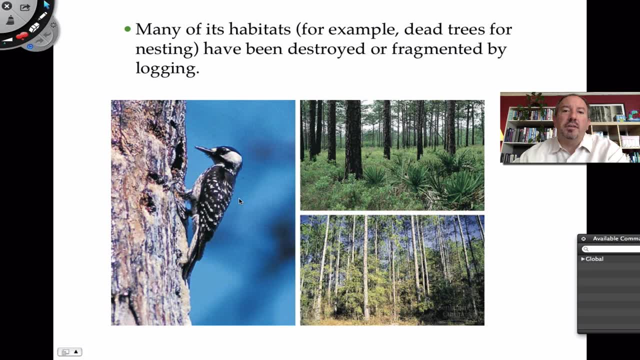 endangered list, And it's really sad, This woodpecker, And so, as it turns out, that many the reason that it's declining because its habitat is destroyed. but it also has some interesting behaviors too, And so it's not as simple as it may seem Like. for example, what's happening is its behavior, the bird itself, 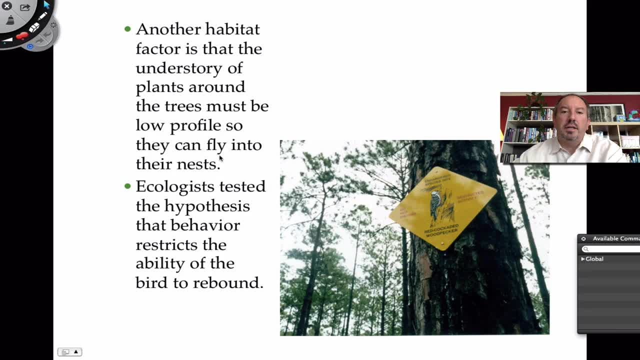 when it flies from nest to nest. as it turns out, it likes to fly very low And as a result of that, there's a lot of fire suppression and there's a lot of low understory, a lot of lower trees. It's. 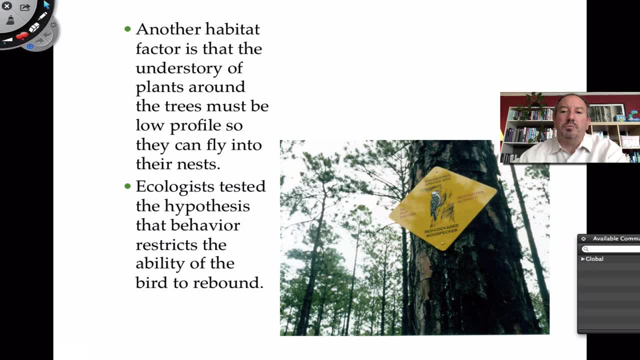 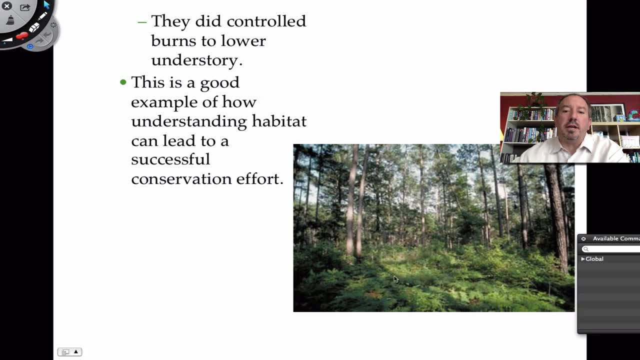 not able to go from nest to nest, And so it's really sensitive. And so what conservation biologists do is they come into the area and test that hypothesis So they burn this sort of understory back, and then they see if the woodpecker is able to manage in this area. And so just, lastly, 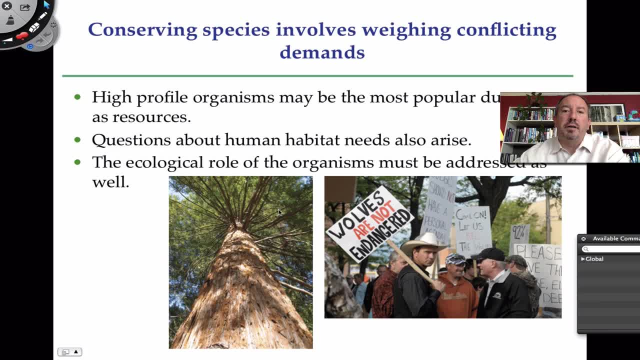 this is the last discussion here and I'm going to show you a little video to finish the video. And so when you're conserving species, it's sort of a balance. You have to weigh the demands Like, for example, real popular species like redwoods are easy to sort of want to save. 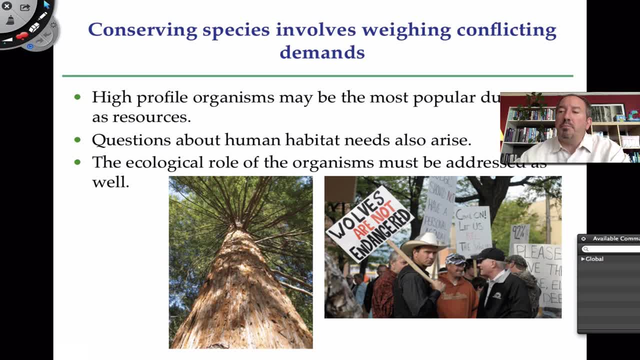 because they're so iconic, like polar bearers and panda bearers and redwood trees, But in so doing and save whales, but it sort of calls the attention to other less known ones, And so it's important to do that. But you have to weigh in the questions about human habitat. 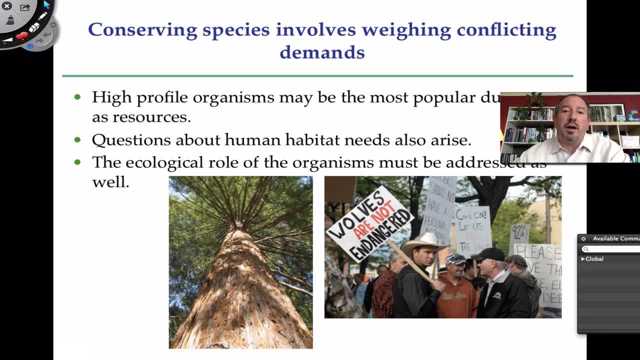 Like we could say, we want to save the gray wolves in Wyoming. But what about the people who are living in Wyoming and their families are endangered by these wolves. And then again, maybe we seek out the organisms to save because of their, their important role. 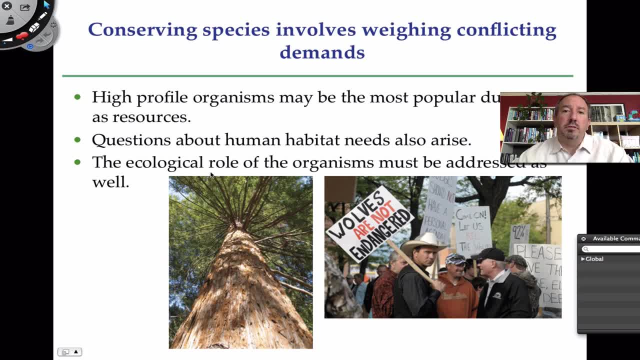 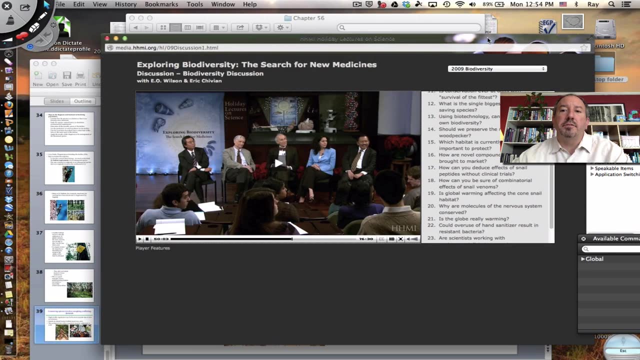 If they're a critical keystone organism, then maybe that's worth saving as well, And so I just wanted to bring that to your attention. And so I want to conclude with a little conversation from the Howard Hughes Medical Institute about those woodpeckers. 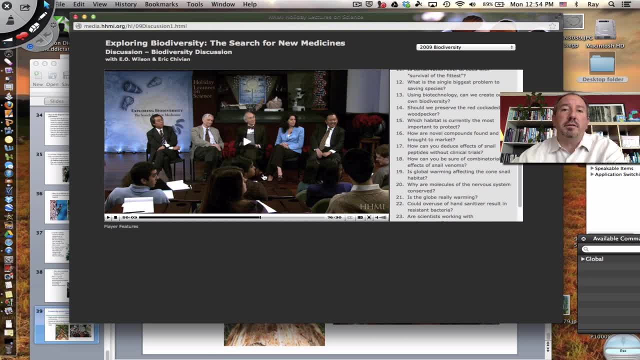 And so this is a panel of scientists that the Howard Hughes Medical Institute assembled to talk about biodiversity, And one of my favorite scientists- actually two of my favorite scientists, actually two of my favorite scientists- Bonnie Bassler and EO Wilson, were on this panel. 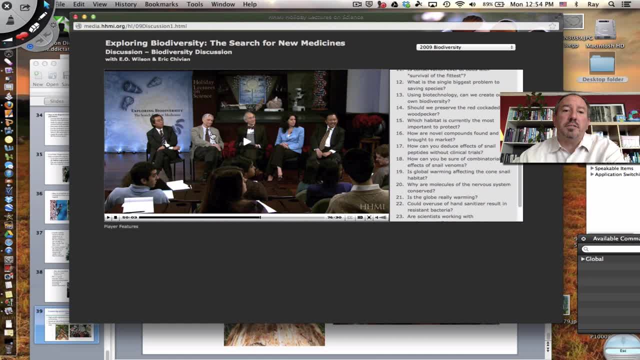 It's really good, And so EO Wilson is addressing this student question from the audience about woodpeckers. I thought you might want to see it to finish the video. A lot of species are really perspicity about their environments. which is why a lot of species are sensitive or endangered or extinct. For example, in Virginia the Red-Hawk native woodpecker lives only in living non in living longleaf pine ecosystems, And the Red-Hawk native woodpecker is basically a species that doesn't really have that much. 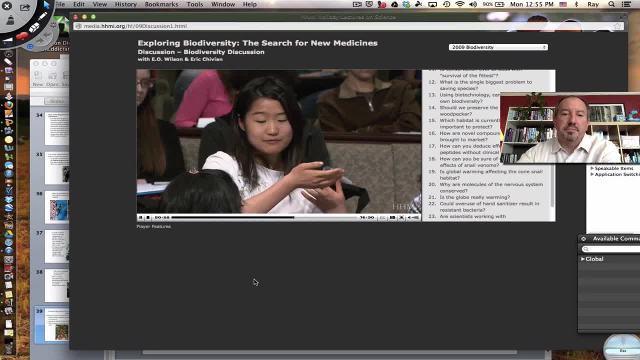 medical potential and isn't the primary food source for any species or anything. So should current non-longleaf pine ecosystems, such as mixed deciduous forests, be converted to longleaf pines to aid the survival of this one species when longleaf pines are homes? 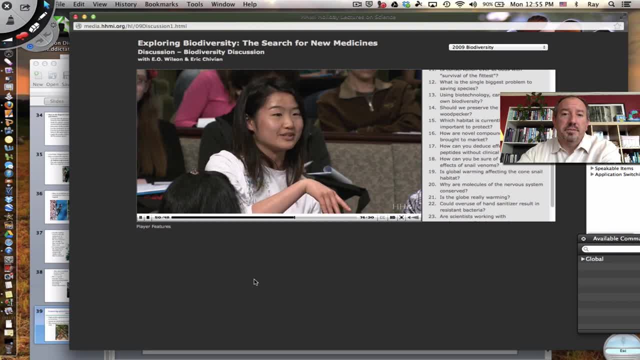 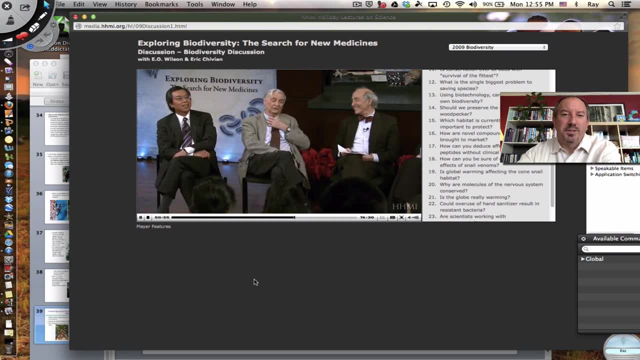 to only a few species, and deciduous forests are even homes to over a hundred species. Oh, I can answer that because I am right now involved deeply in that woodpecker in that forest. Yes, We're talking about the red-cockaded woodpecker, which is an endangered species and once and was found from the Carolinas to Texas in the longleaf pine savanna forest, which was covered 60 percent of the southern United States, And between the Civil War and the turn of the last century we cut it all down so there was less than one percent of old growth, original old growth, left. The red-cockaded woodpecker depended on old growth of longleaf pine to nest, and so it went down. It almost became extinct, just as the ivory bill woodpecker became extinct in 1944 when we had cut down. Cut down all of its trees that it needed, which were old growth cypress and a few other. 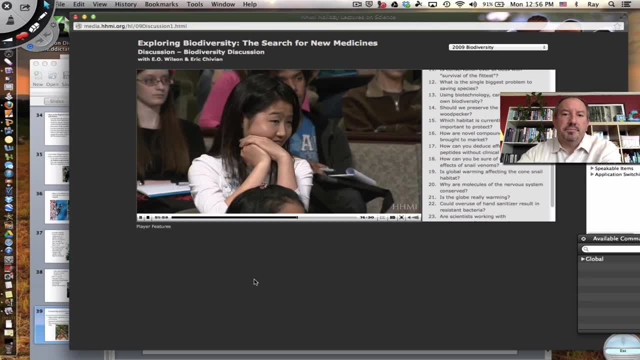 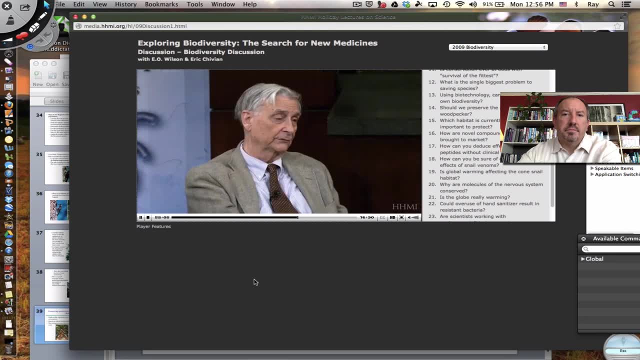 giant trees in the floodplain forests, the swamps of the south. We lost that one. We're not going to lose the red-cockaded woodpecker and it is not a trade-off, quite the opposite, Because, in addition to the red-cockaded woodpecker, dependent on that great at once great ecosystem,